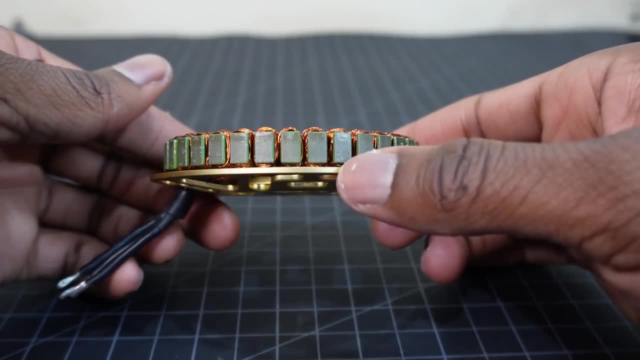 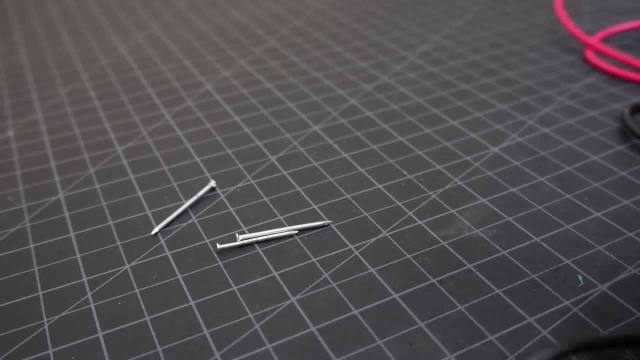 phases of the motor. This motor is made of copper wire, which makes up the three phases of the motor. this motor has 36 coils, or 36 slots, If you remember from physics class. a coil of copper wire can create a magnetic field when current flows through it. 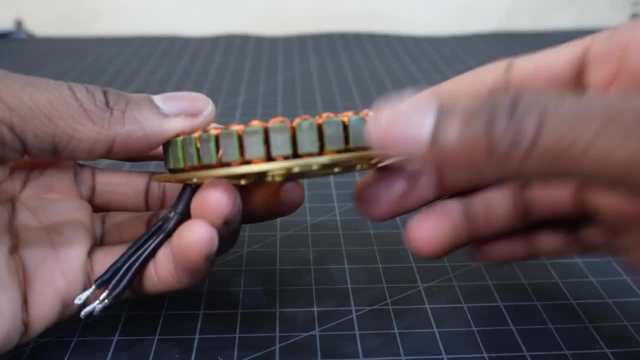 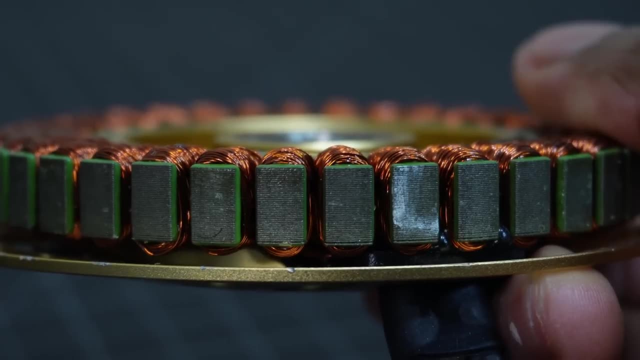 This is called an electromagnet or solenoid. The stator of the motor itself is made up of laminated silicone steel sheets stacked on top of each other with thin insulation in between. This is a key component to the motor design. Steel, being an iron alloy, is ferromagnetic. 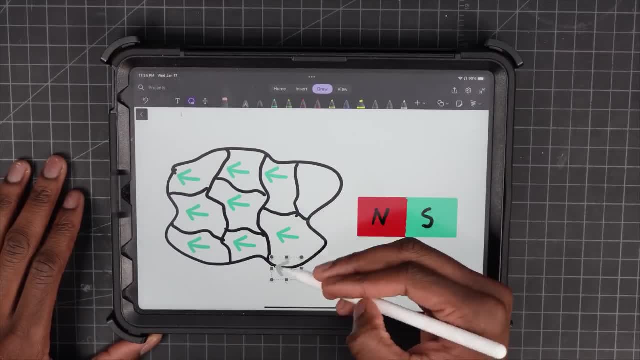 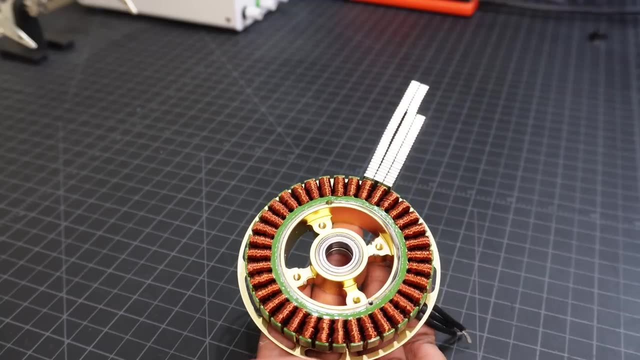 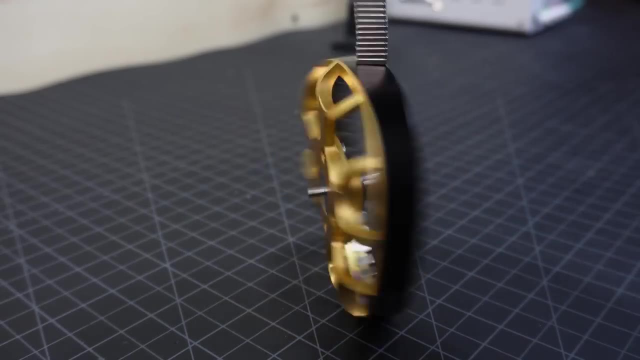 which means that it becomes magnetized in the presence of an external magnetic field. With this ferrous core, the magnetic field of the coils is magnified, which makes the motor more powerful. This same advantage is applied to the rotor as well. The ring on the rotor is made from steel, which magnifies the magnetic field of the permanent 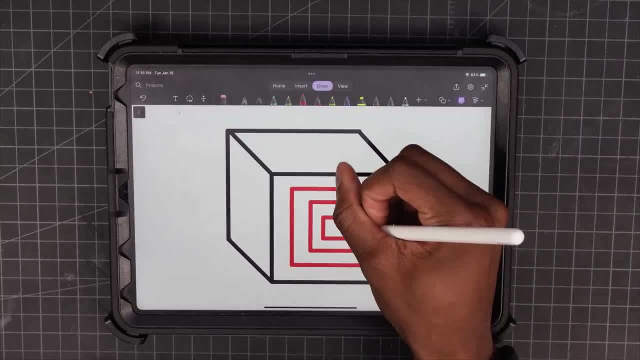 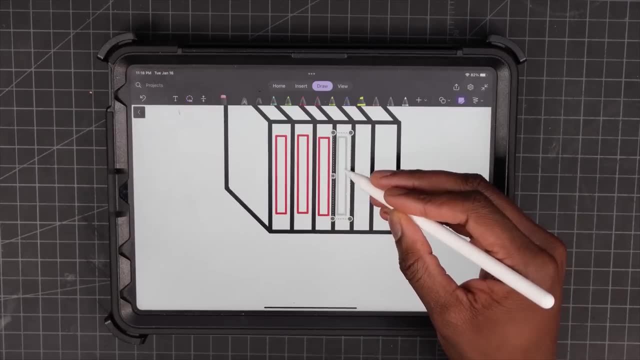 magnets. Now, the reason that the stator is made from stacked sheets instead of just a chunk of steel like this is because stacking the sheets breaks up the eddy currents, which prevents energy loss from heating. These eddy currents are caused by the changing magnetic field of the coils. 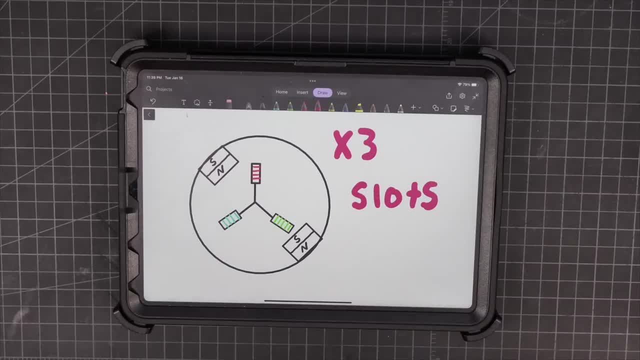 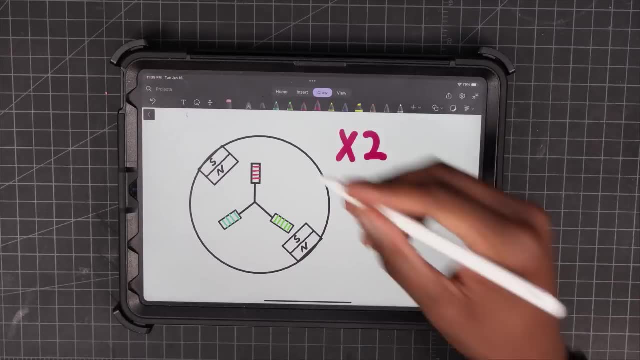 The most common problem facing motors is that on any motor, the total number of slots is always a multiple of 3 because the motor has 3 phases, and the total number of poles is always a multiple of 2 because you can only have 2 poles, north and south. That would make this the most basic brushless. 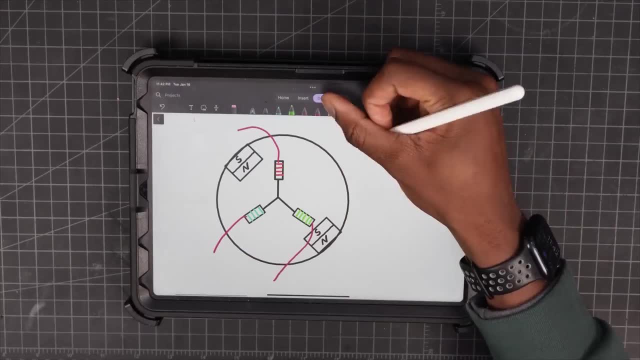 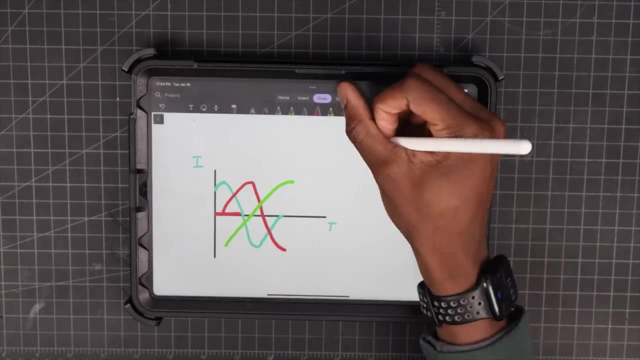 motor that you can make. If you were to spin a brushless motor and monitor it on an oscilloscope, you would find that each phase outputs voltage in a sine wave, with each phase being offset by 120 degrees. This is also known as three-phase AC. 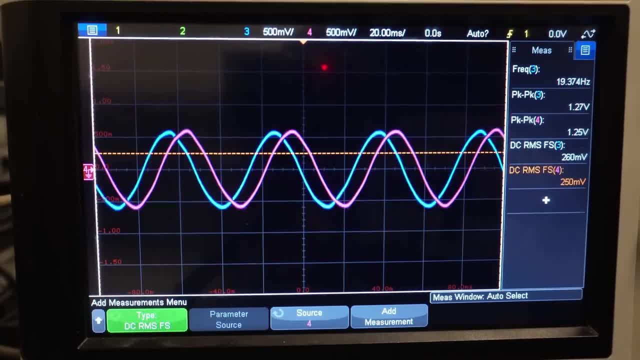 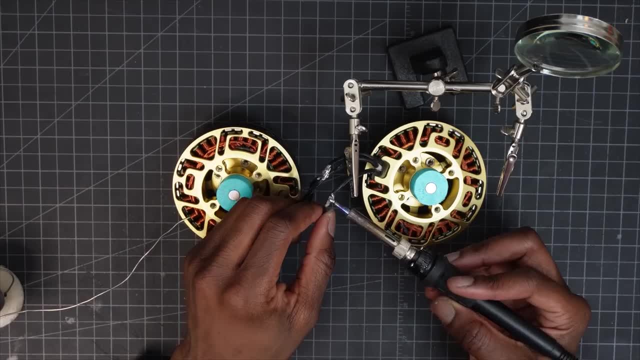 tried this using an oscilloscope at my university. you can only see two waves because i had to use the third phase of the motor as ground, so you'll just have to trust me on the third one, since a motor can also act as a generator. if you have two brushless motors, you can make one drive the other. 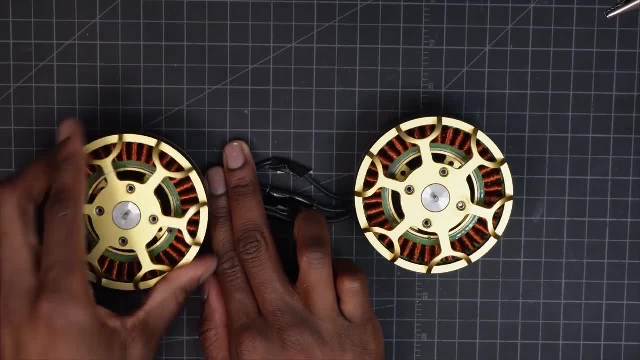 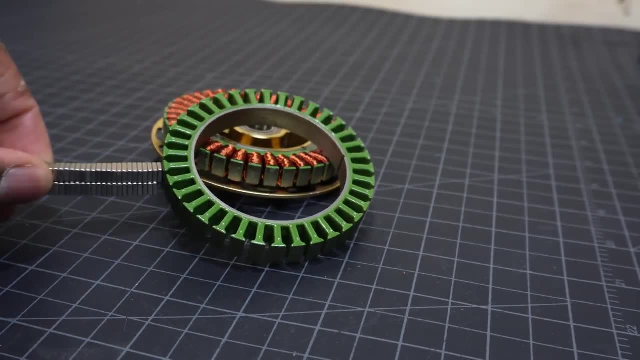 which is pretty neat, and with that let's build the motor that we're going to use for the actuator. i want the motor to have 40 poles and 36 slots, which is the same as the eagle power, so i bought a similar size stator from aliexpress. this one is 81 millimeters in diameter. the plan is to 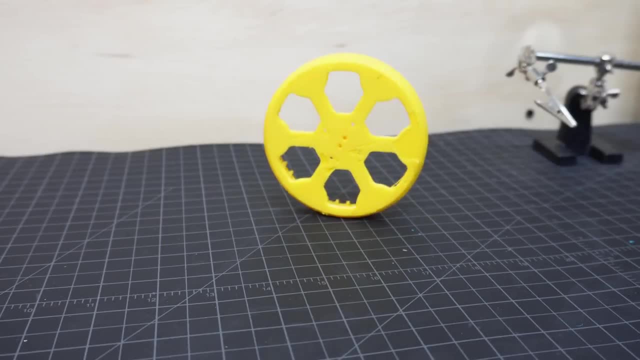 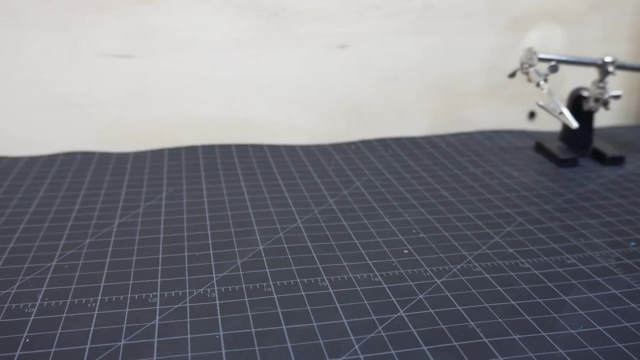 eventually machine the rotor out of steel, but for proof of concept, i just 3d printed it for now. i bought these cheap 10 by 5 by 2 millimeter magnets from amazon and i'm going to glue them to the rotor in alternating polarity using some jb weld epoxy, something that i found out while 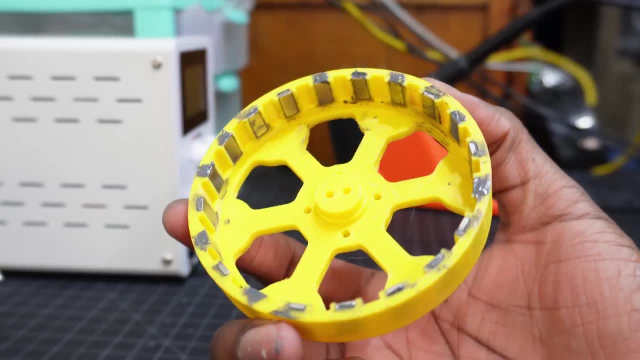 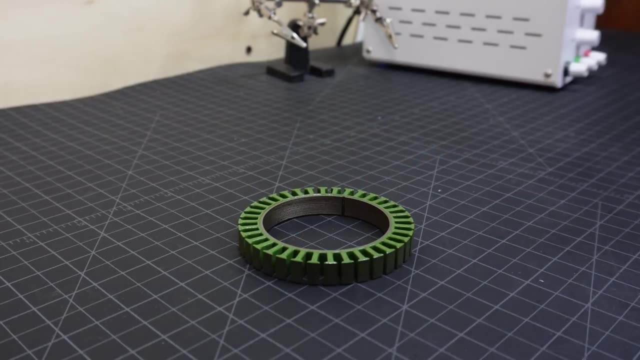 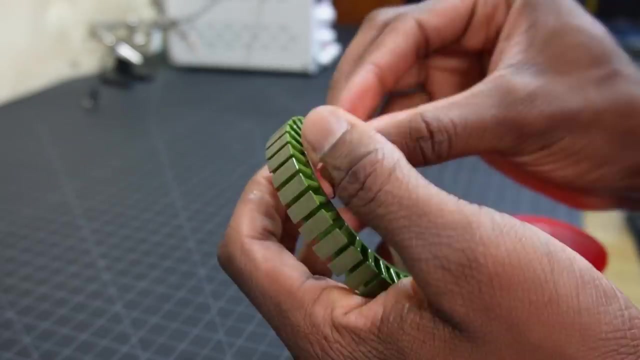 gluing the magnets is that jb weld is 11 steel, which means that it should actually enhance the motor's performance, though probably not by a lot. i'm going to be using 22 gauge enameled copper wire to wind the stator. these windings are done in a specific pattern, depending on your slot and pole configuration. 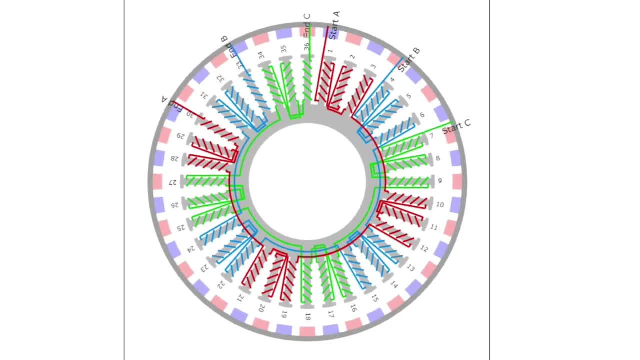 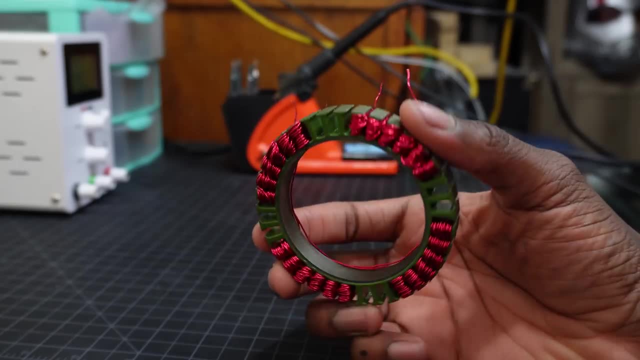 i used this website to figure out my winding pattern, which i'll link below. i got about 17 turns on each slot and, side note, winding this stator took several hours to complete and most definitely gave me arthritis. if you ever plan on doing this, my recommendation is that you 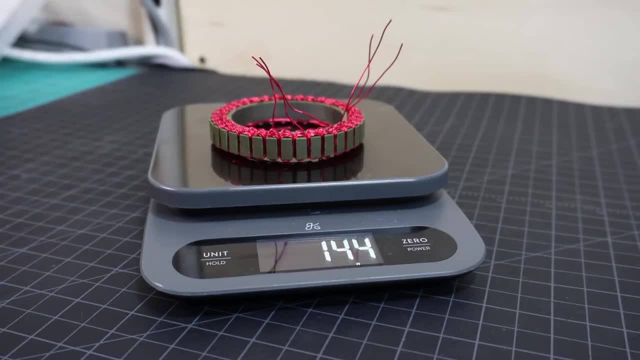 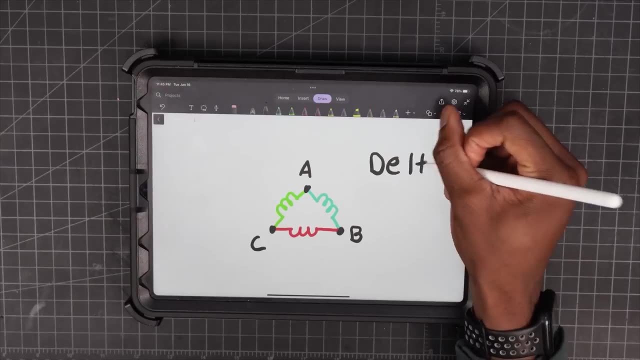 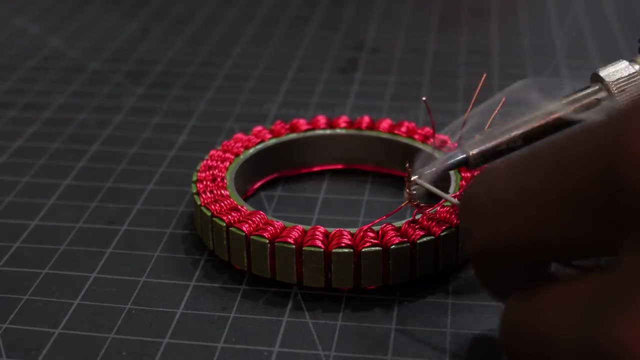 don't? the phases of the motor can be connected in two different ways. in star configuration, the phases all share a neutral point. in delta configuration, the phases are essentially in series. i'm going with star configuration because it looks like that's what the eagle power uses. now, after spending all that time winding the stator, i found out that it would be just too. 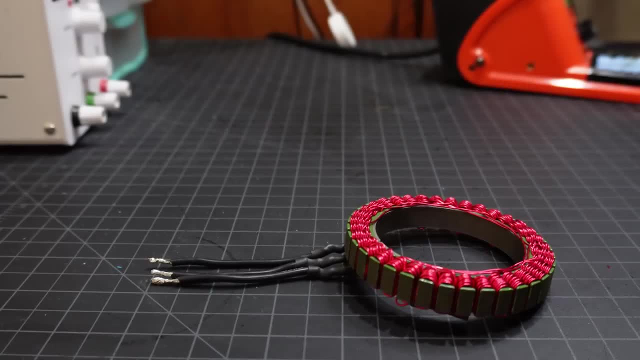 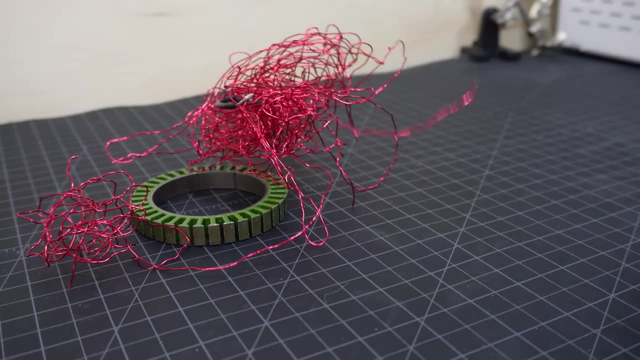 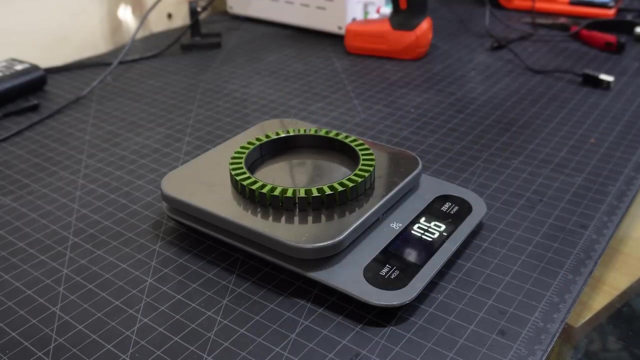 small for the actuator design that i had in mind. so there goes five hours of my life anyway. i decided to buy a bigger stator that is 100 millimeters in diameter. as well as being compatible with my design, it should give me more torque. this time i decided to use 26 gauge copper wire, which is much thinner and should get. 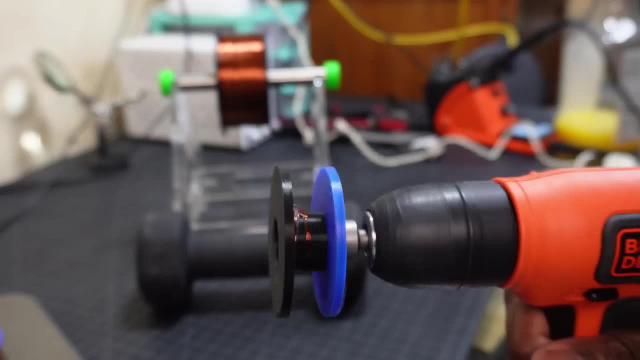 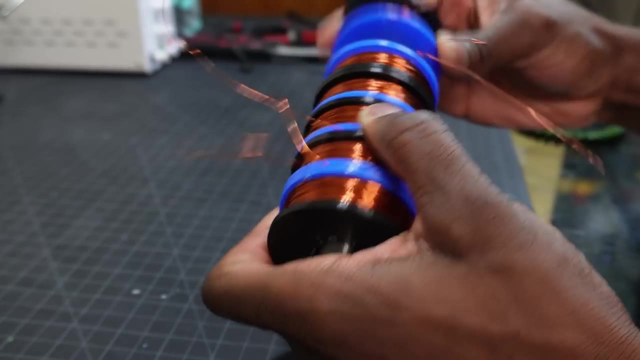 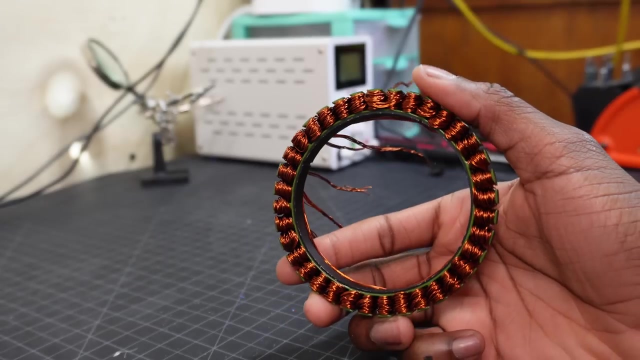 me more turns per slot. since the wire is very thin, i decided to divide the roll into six mini rolls and wind the stator with six strands of wire. i did six turns of the six strand wire on each slot, making 36 turns per slot. doing it this way also made the process slightly less painful. i also 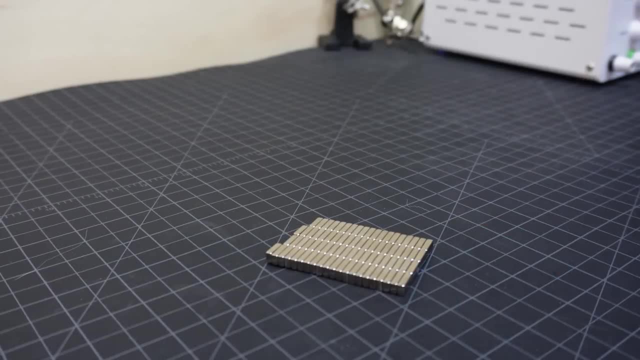 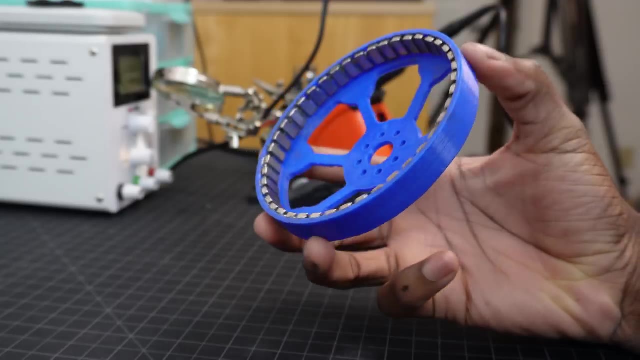 3d printed a bigger rotor for the stator. to be able to wind the stator in the right direction and use slightly bigger but still cheap 10 by 5 by 3 millimeter magnets with a bigger rotor diameter, i decided to use 42 magnets instead of 40 magnets, making a 36n 42p configuration. 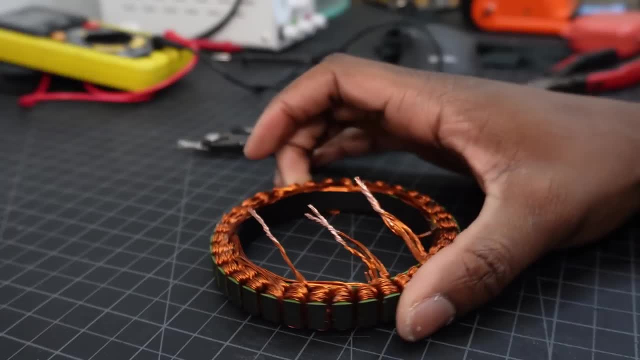 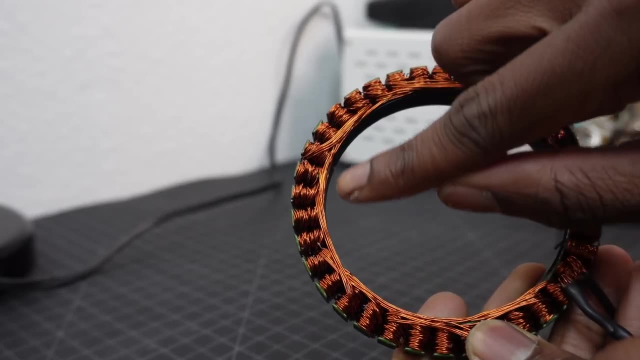 and after winding this stator, history repeated itself. i realized that i was going to have to fit a gearbox in the center of the stator, which could not be possible since there were strands of copper wire overlapping the center, which created just enough of an inconvenience for nothing to fit in snug. 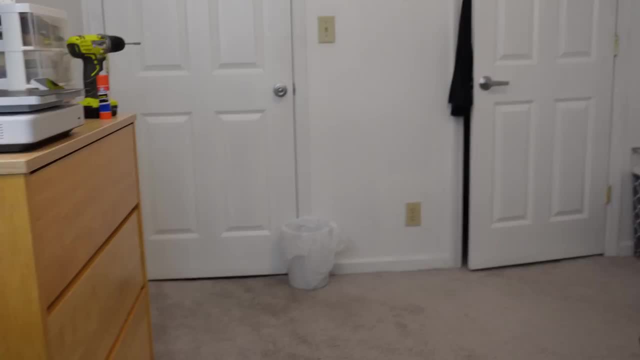 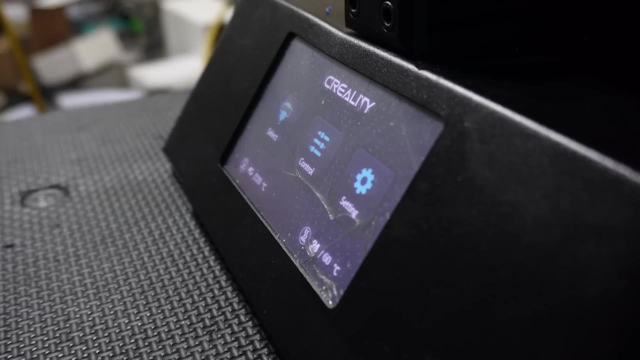 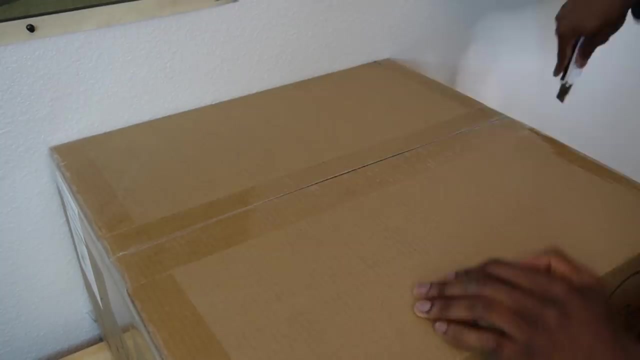 in the stator. now, on a more positive note, while making this video, i bought a new 3d printer. pro tip: if you ever find yourself designing parts that don't exist to make your printer work, it may be time for a new one. i bought a bamboo lab a1 and it's awesome. they. 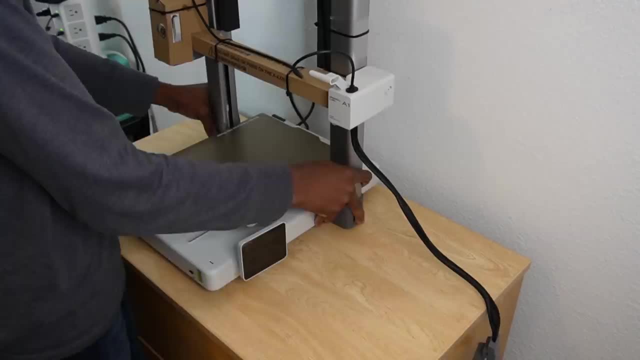 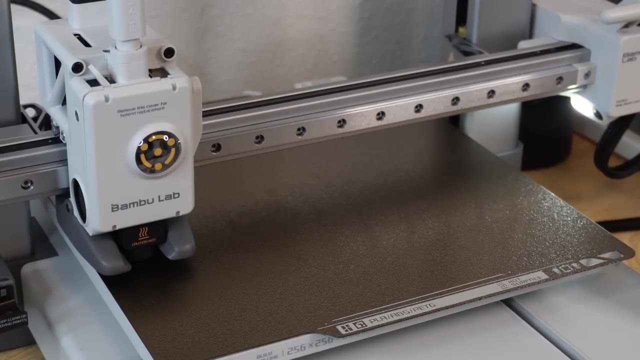 aren't paying me to say this. i just really like this printer. or maybe it's just that my old printer was so bad that anything slightly better is an upgrade. that's besides the point. this can determine the flow rates of different filaments, which gives really smooth prints. 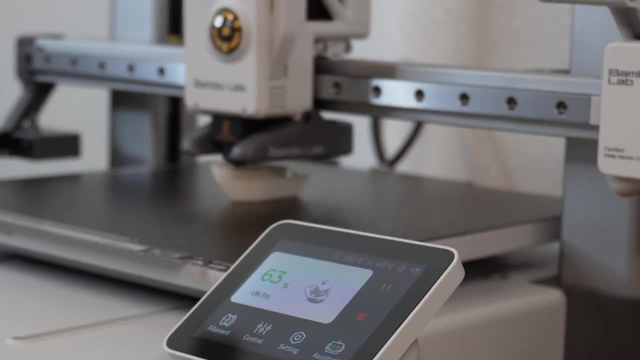 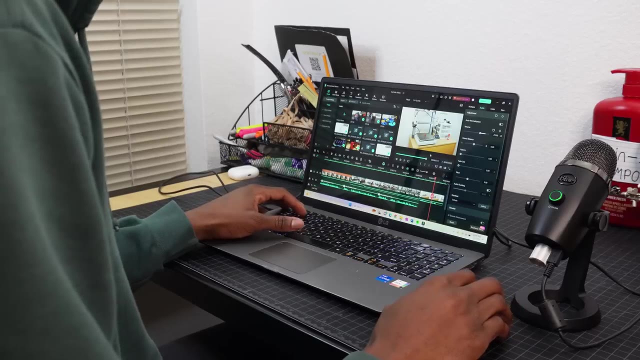 It's also extremely fast, but in my opinion, the best feature is this sick tune that it plays after each print. Quick FYI: while editing this video, I got an email saying that this printer had been recalled due to a cable issue in the heated bed. 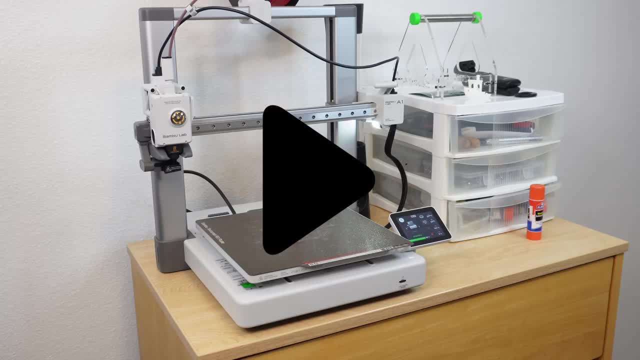 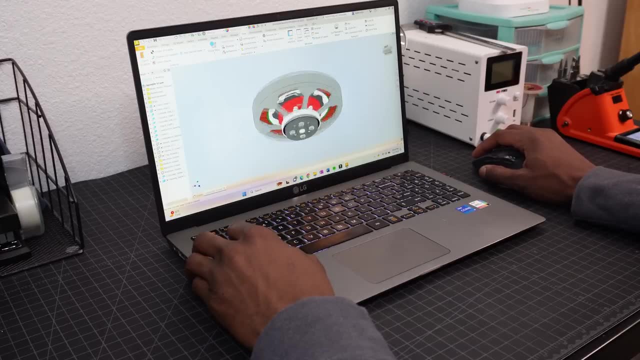 Isn't that just absolutely fantastic? Anyway, back to the video. I figured that the best plan of action was to sit down and design the actuator, so that I knew exactly how to build the motor. A big part of this process was designing the gearbox. 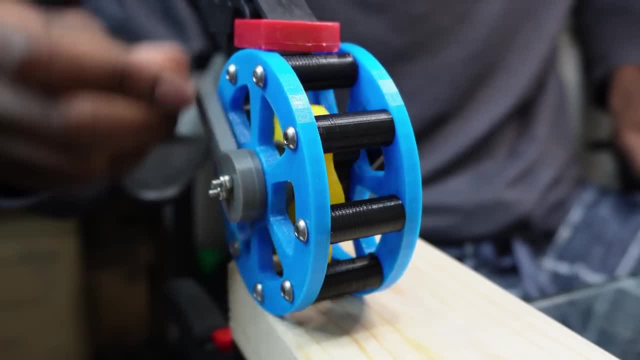 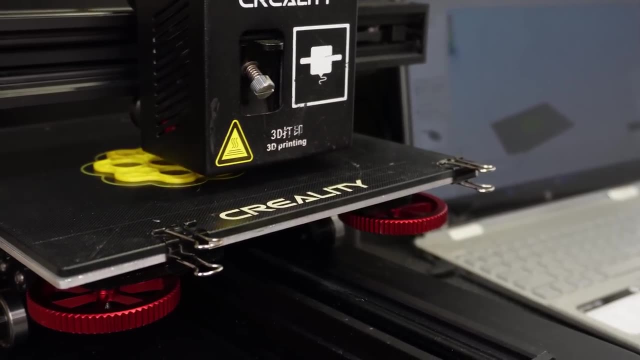 As mentioned before, I'm going to be using a cycloto drive, or as I call it, wobble drive, And since the gearbox is going to be baked into the motor design, I'm calling this an internal cycloto actuator. The main body of the gearbox is a fixed ring made up of these roller pins. 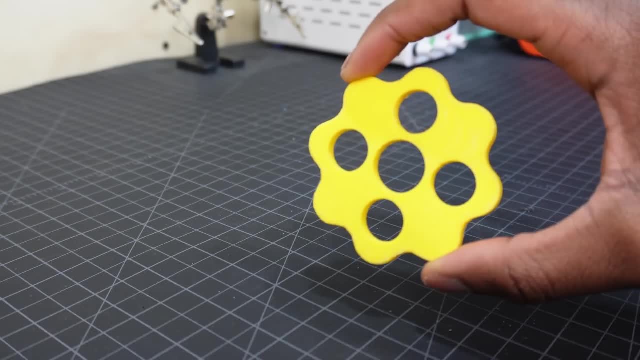 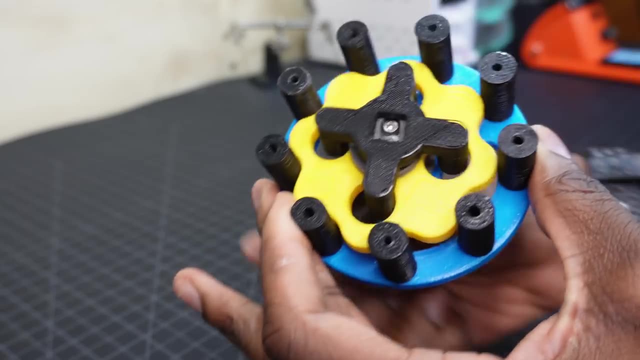 You then have this eccentric shaft, which is off-center so that the cycloto disc can roll over each roller pin. The gear reduction is then captured by this output shaft and the gear reduction is equal to the number of lobes on the cycloto disc. 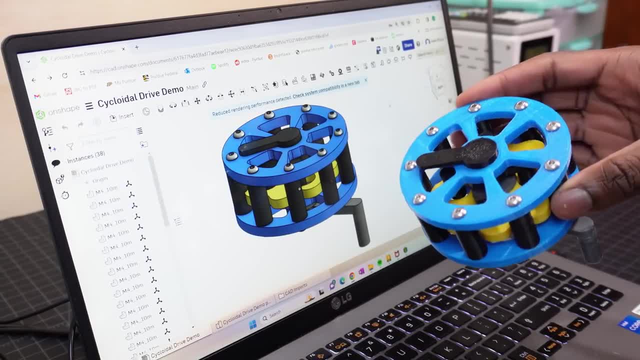 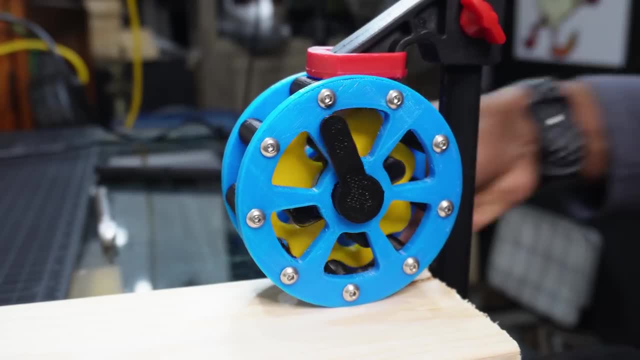 Here there are 9 roller pins and 8 lobes on the disc, making an 8 to 1 gear reduction. Now there is one problem: Since the disc is off-center, the gearbox isn't balanced, which could lead to lots of. vibration. Imagine you held a weight in one of your hands and tried to spin To balance yourself out. you would need to add a weight to your other hand, But it doesn't matter, Because you'll be depressed either way. The same applies to the cycloto gearbox. 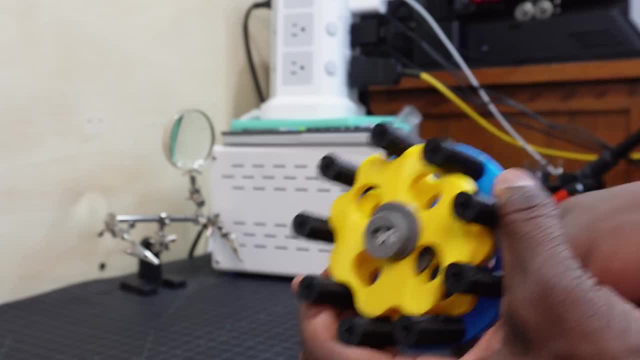 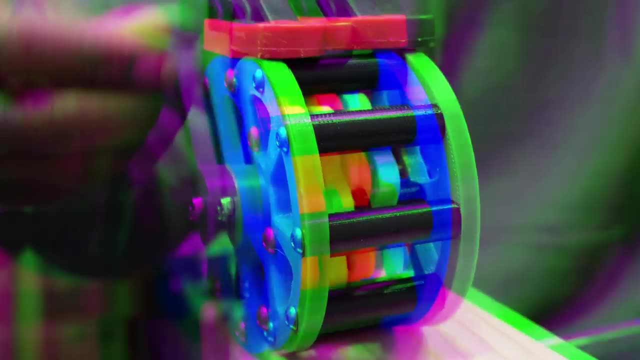 Not the depression but the counterbalance. If we just add on another disc that's 180 degrees out of phase with the original disc, then the gearbox should be perfectly balanced, As all things should be In my opinion. cycloto drives are quite interesting. 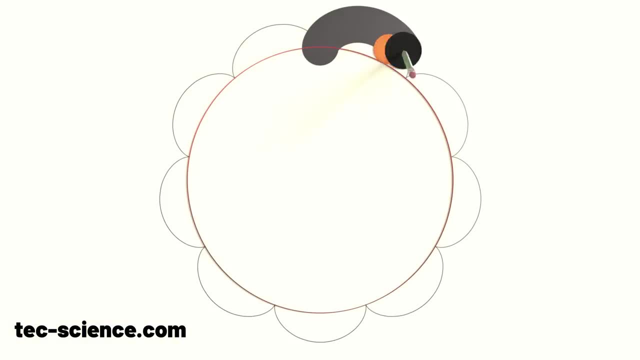 The shape of the disc is made by rolling a smaller circle onto a bigger circle and tracing out the path of one of the points on the smaller circle. To do this in CAD I just used equation driven curves. I'm not going to go into too much detail on this. 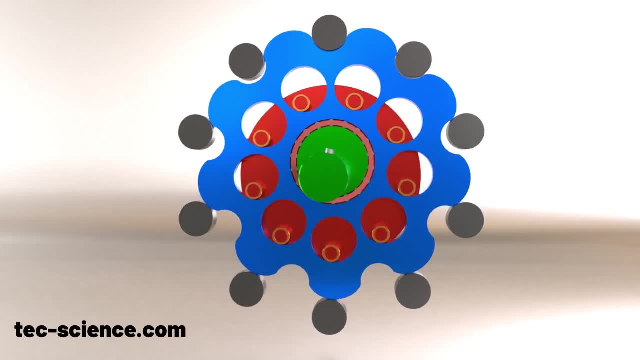 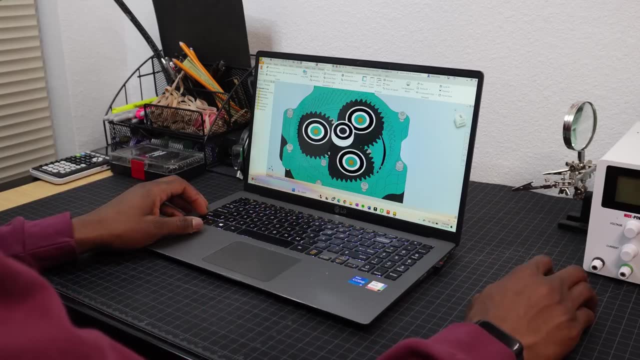 I'm just going to show you how to do it. The first thing about cycloto drives is that the disc maintains contact with each roller pin at all times, which means virtually zero backlash. This is something that can't be said for planetary gear sets. 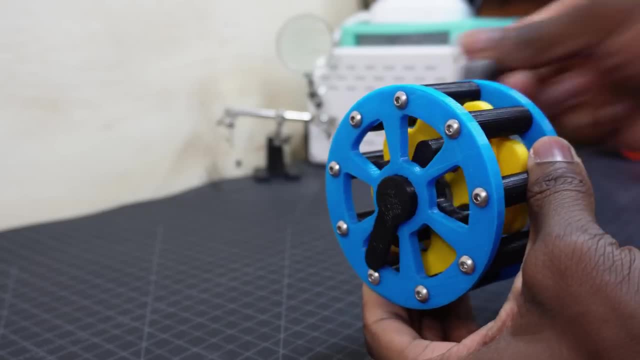 Best of all is that with cycloto gearboxes you can make pretty much any gear reduction that you want in the same amount of space. Now, just like the example gearbox, I want the reduction of my actuator to be 8 to 1,. 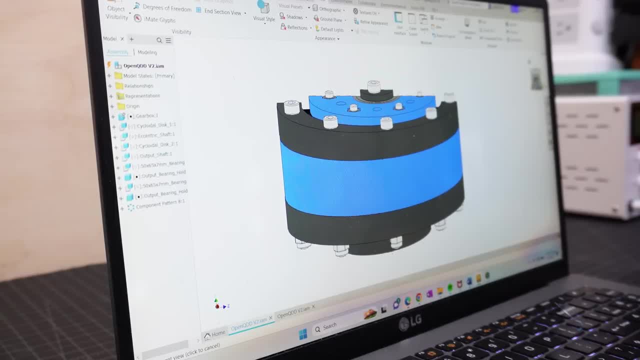 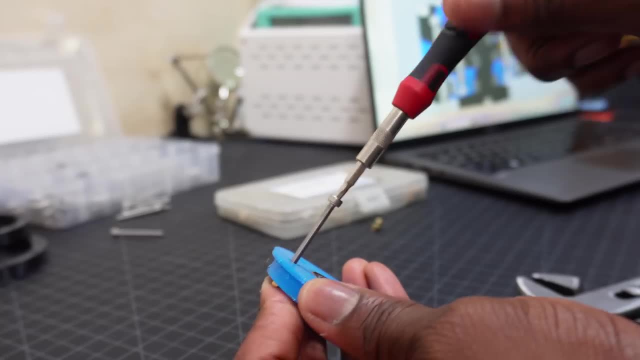 since quasi-direct drive actuators generally have reductions under 10 to 1.. I started by designing a cycloto gearbox to fit in the center of the stator and then worked on building a prototype. Making this design was a bit tricky. I had to go through several iterations to get it right. 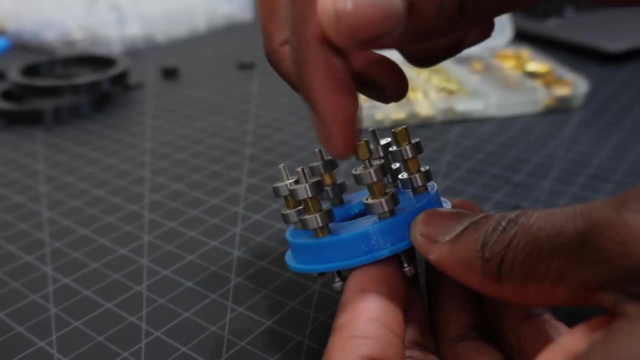 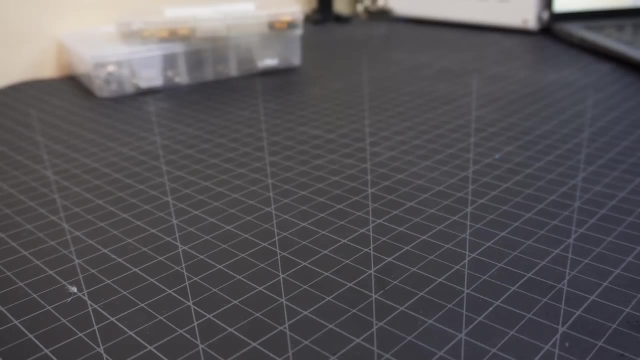 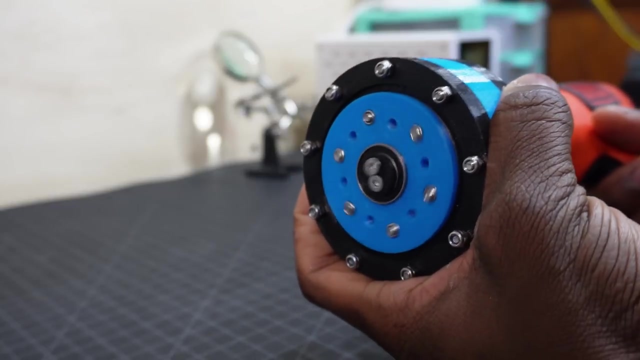 The main goal was figuring out the smallest screws, bearings and spacers that I could use without compromising the actuator's strength. I genuinely spent weeks getting the design to this point, But once everything was built, it worked pretty well. I'm also glad to see that it's backdrivable, which was one of my main concerns with the 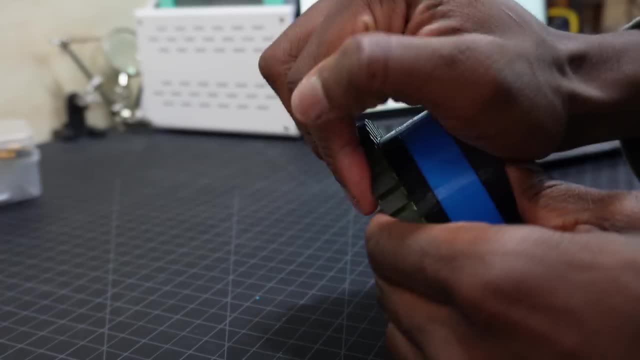 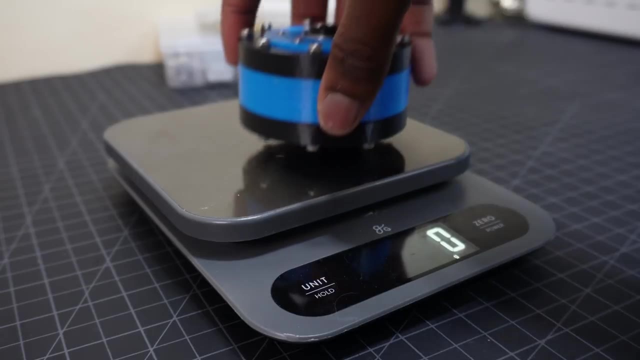 design As planned. it fits right into the center of the stator. Now that I know that the gearbox works, it's time to get some parts machined for the final actuator, which brings us to today's sponsor, PCBWay. 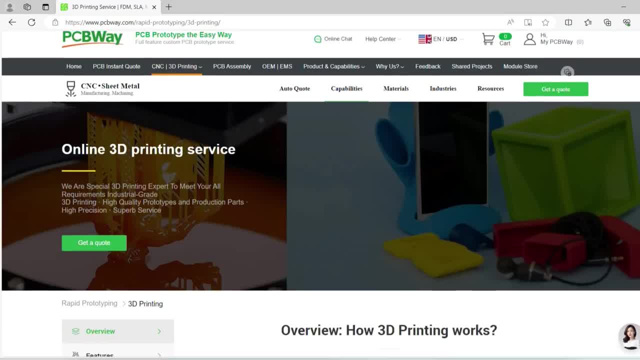 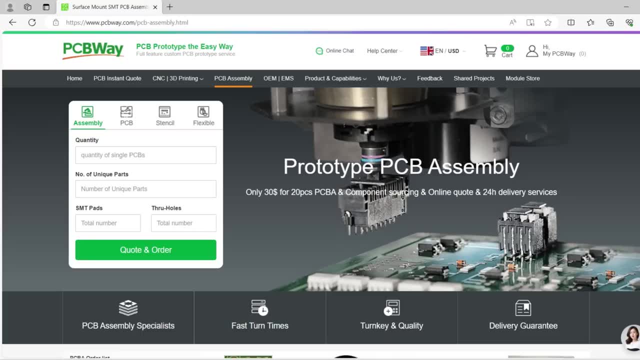 PCBWay is an online service for all of your machining needs, from 3D printing to CNC machining, to sheet metal fabrication, injection, molding and, of course, PCB making. I wanted to get the rotor of my motor and the fixed ring of my gearbox CNC machined. 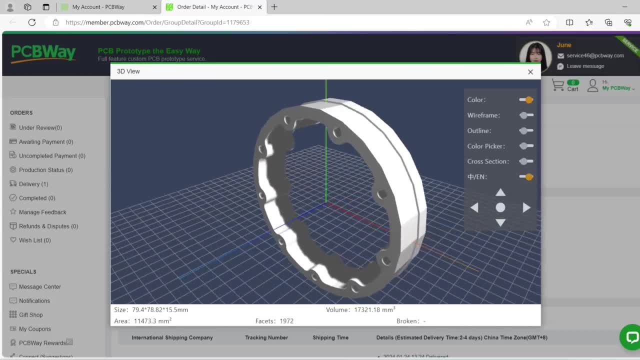 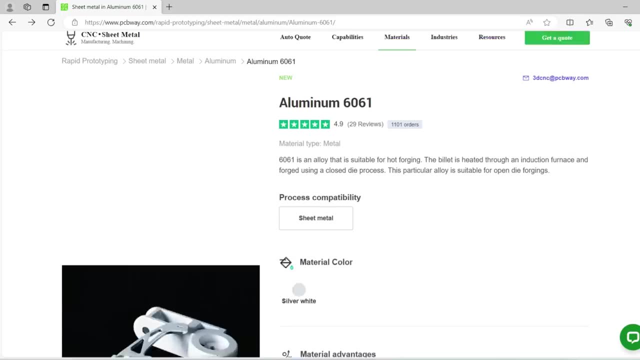 and after uploading my files to the site, I was able to get the motor and the fixed ring of my gearbox CNC machined. I could choose among a variety of materials that PCBWay has to offer. I ended up choosing mild steel- 1045- for the rotor and aluminum 6061 for the fixed ring. 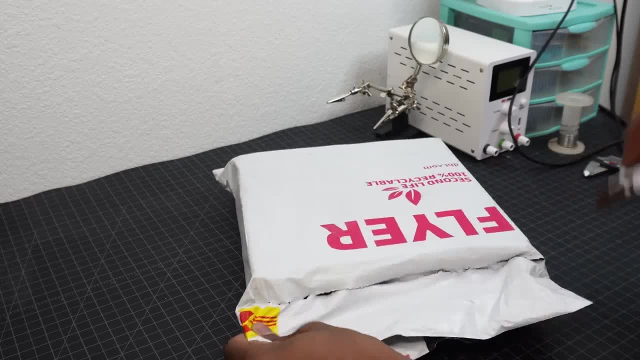 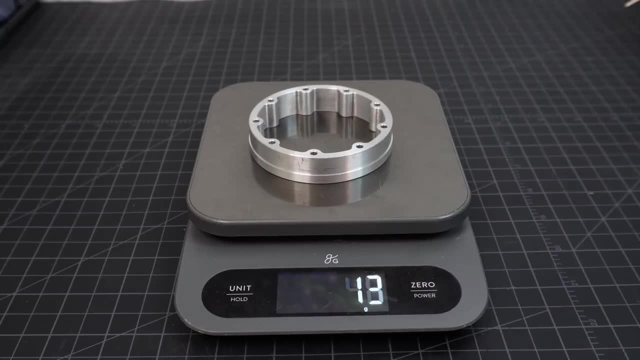 After that, I received a quote almost instantly and then placed my order and got my parts 10 days later. I mean, just check out how nice these came out. Here's the fixed ring and here's the rotor. Don't let your access to machining hold you back from making your projects. 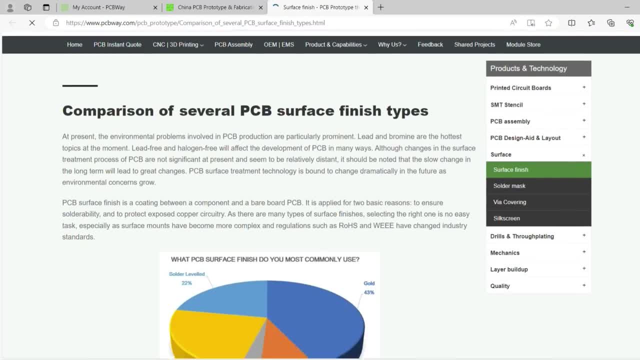 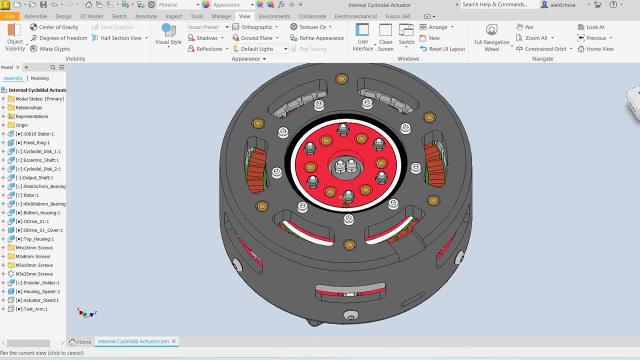 Head on over to PCBWay and take a look at their multitude of resources to figure out what's best for you. You can check out PCBWay today by going to the link in my description. Alright, so now that we have the metal parts, it's time to assemble everything. 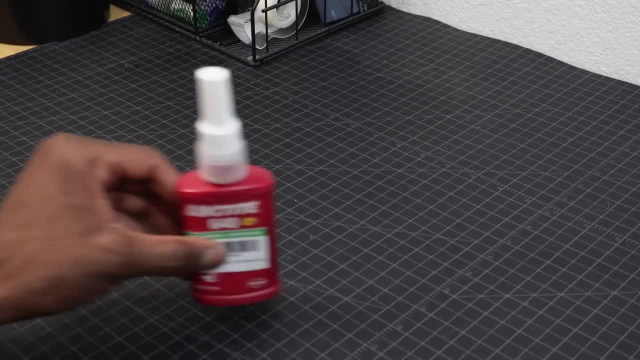 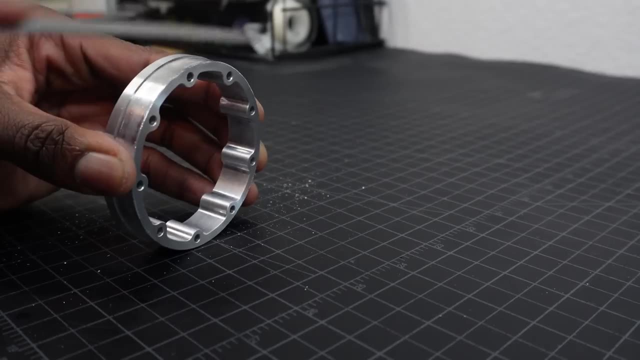 I'll first work on the stator. I'm going to be gluing the fixed ring to the inside of the stator using Loctite 648 Retaining Compound. It's going to be a press fit, but I may have overcompensated a bit, so I'm going to need 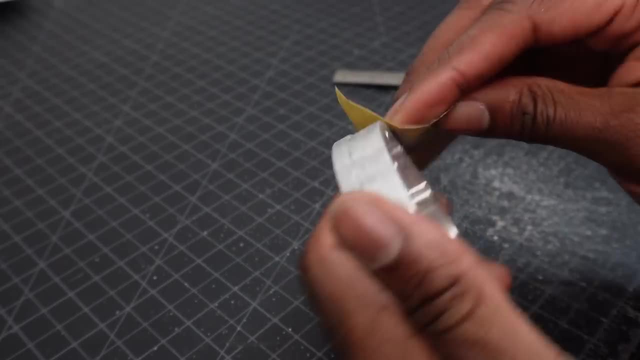 to sand it down. This isn't the right way to go about it, but a file and some other stuff will do. I'm going to use a piece of wood to glue the fixed ring to the inside of the stator using Loctite 648 Retaining Compound. 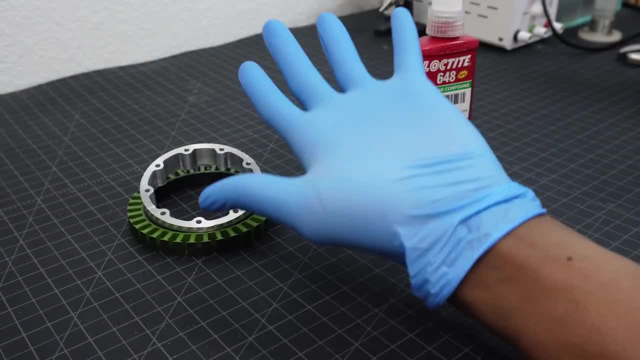 I'm going to use a piece of wood to indeed glue the fixed ring to the inside of the stator using Loctite 648 Retaining Compound. I'm going to also grind and sandpaper. the 줄 to cover it Actually, is all I had on hand. 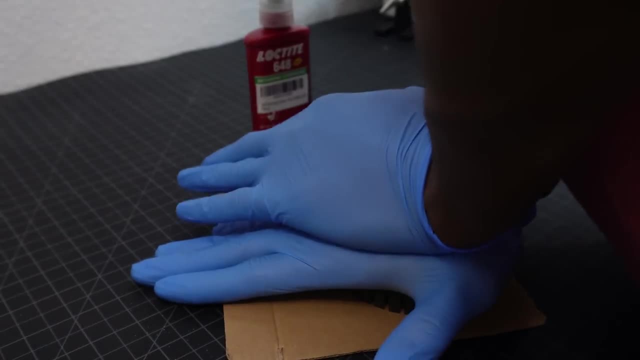 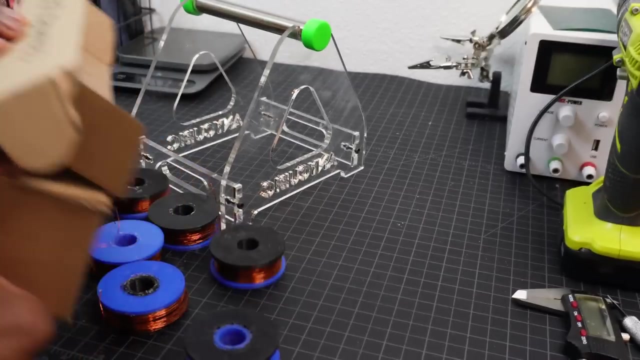 Eventually it fit, and I added Loctite to prevent it from being twisted out of line. Once that's dried, it's time to coil the stator- Hopefully for the last time, but knowing myself probably not. Once again, I'm using about two strands of wire to do 6 turns on each slot, which is 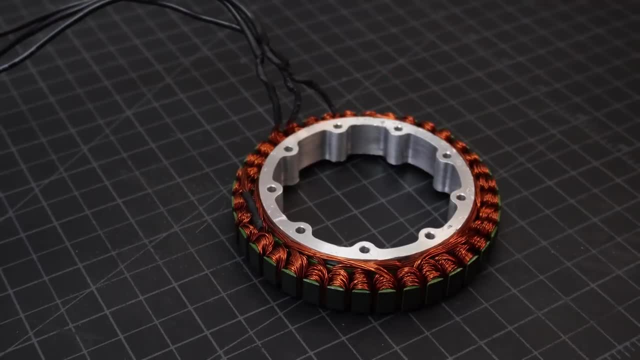 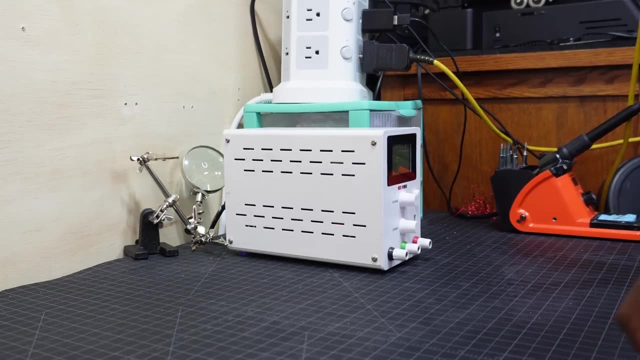 essentially 36 turns per slot. Now it's time to work on the rotor. This time I'm using really strong 10x5x3 mm and 6mm audio card Christmas car secretly- Sierra n52 grade magnets. these aren't your regular fridge magnets. like before, i'm gluing the magnets to the 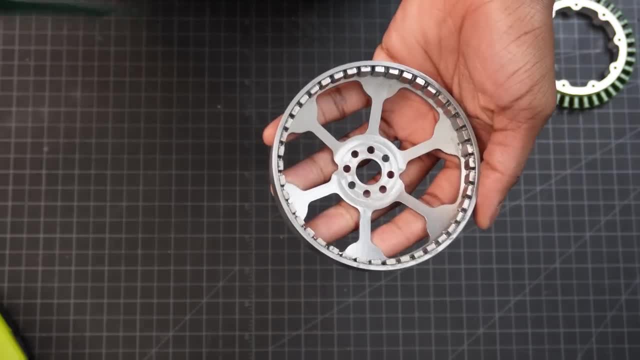 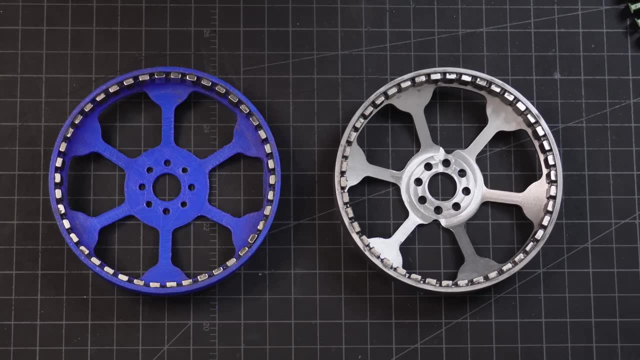 rotor with jb weld in alternating polarity. i have this magnetic viewing film that allows you to visualize a magnetic field. i can use this to check if any of the magnets are weak. here you can see the difference between the fields of the 3d printed rotor and the steel rotor. the magnets on. 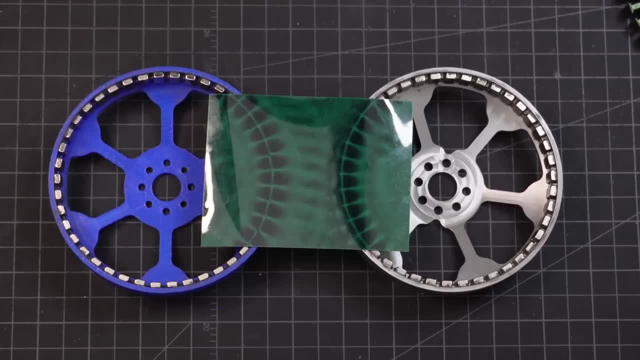 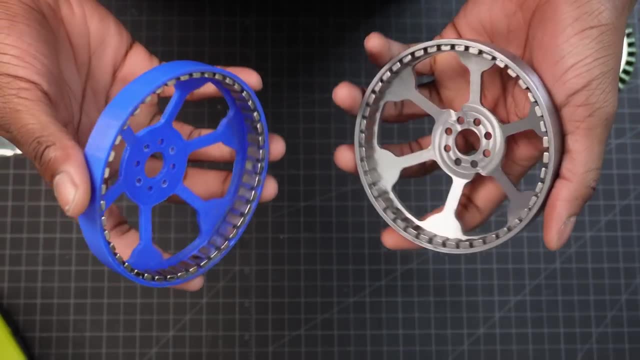 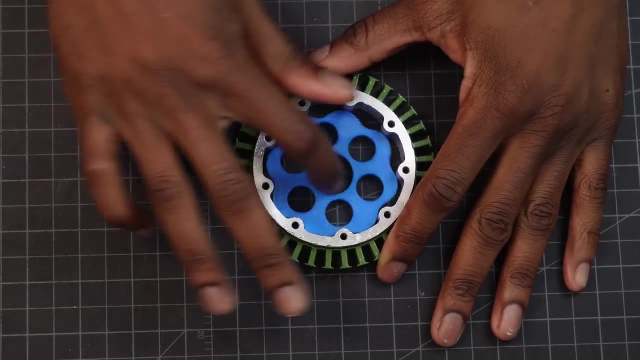 the steel rotor have a higher magnetic field concentration pointing inwards, which means more flux, less speed, higher torque and higher efficiency. this is why dc motors have a flux ring. seeing something that i designed become realized in metal for the first time was quite amazing. with the rotor and stator built, i think it's a good time to build a mock motor. 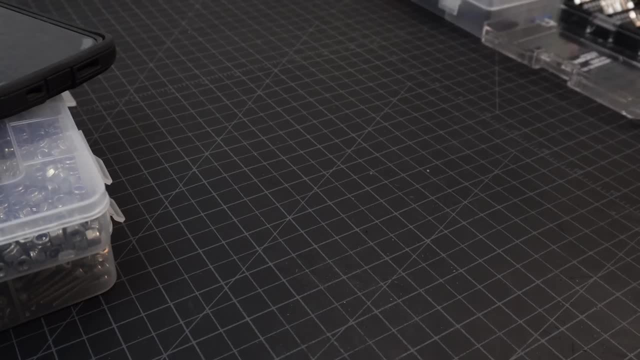 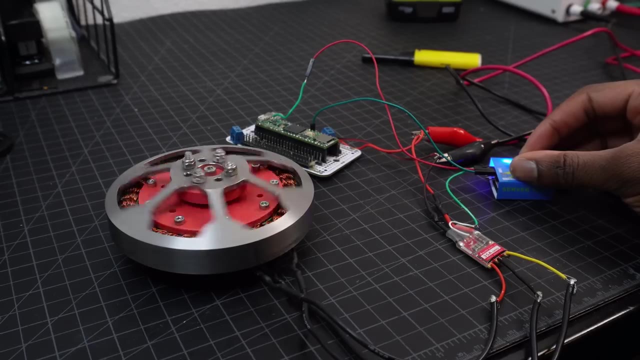 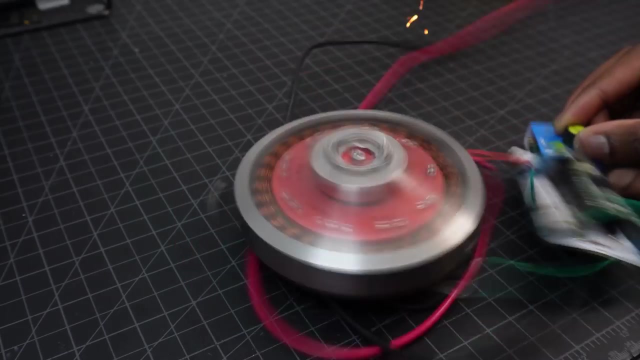 because there's a good chance that i winded the stator incorrectly. to test it out, i'm using an esc and a speed controller knob and, to my great surprise, it actually worked. by the way, that clip that you saw from the beginning of the video was the inertia of the motor causing 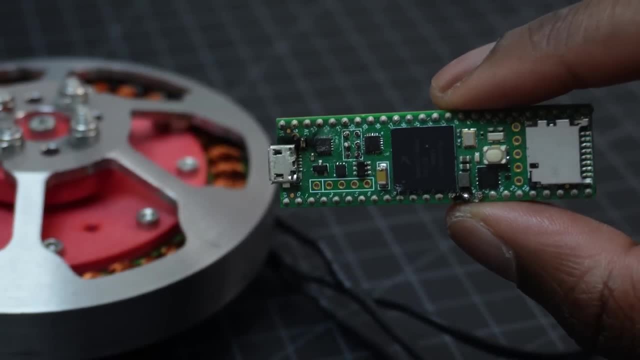 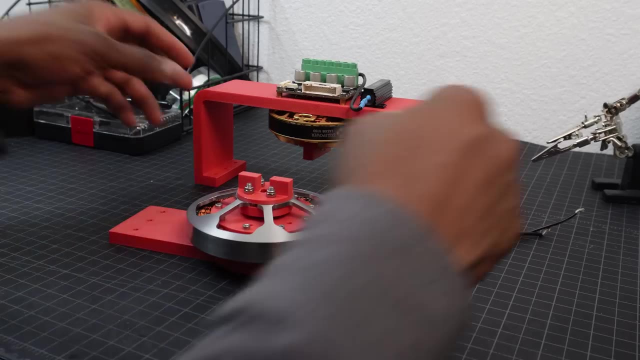 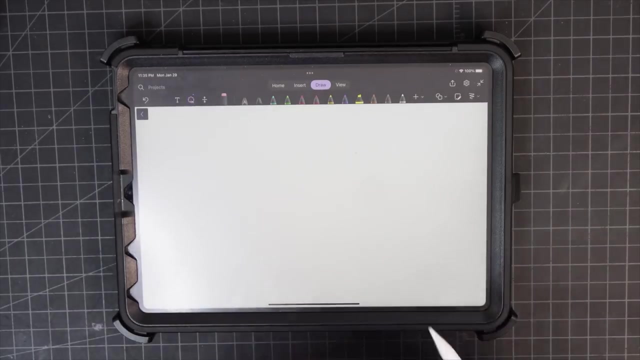 a short which ended up burning the microcontroller that i was using as a 5 volt regulator. this is your reminder to always clamp down high speed spinning objects. i also went ahead and determined the kv rating for the motor. kv is essentially the rate of rpm per volt of a brushless motor. the eagle power is rated for 90 kv, which means that it'll spin. 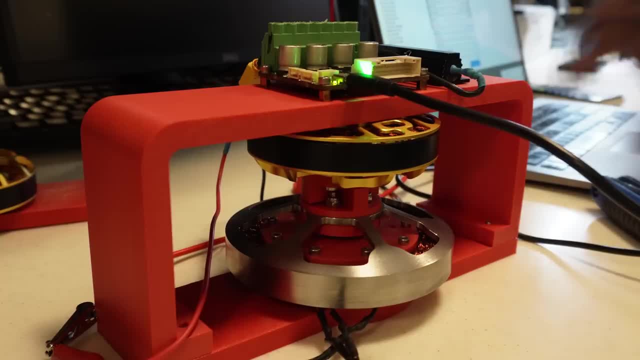 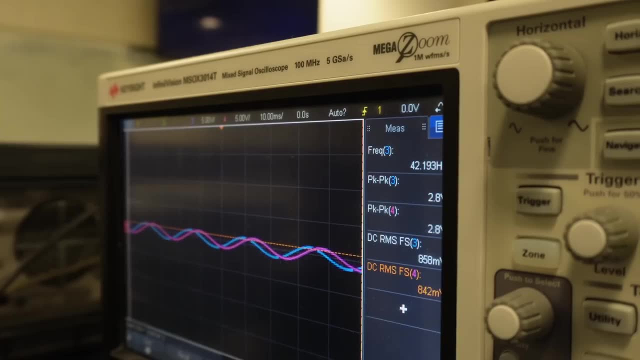 at 900 rpm if 10 volts is applied to it. for the test setup, i have the eagle power motor spinning my motor at 300 rpm. i'll then read the rms voltage of one of the phases on an oscilloscope. after doing some calculations, i found that the kv rating for the motor was 104. 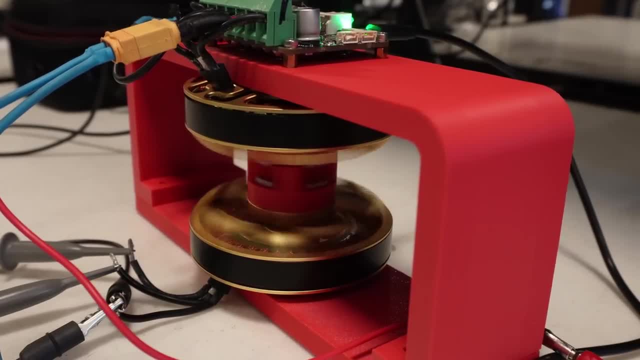 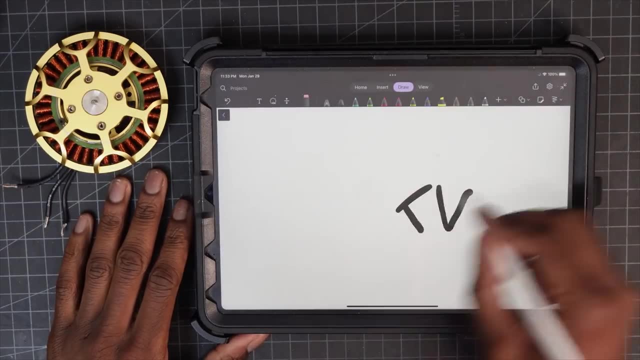 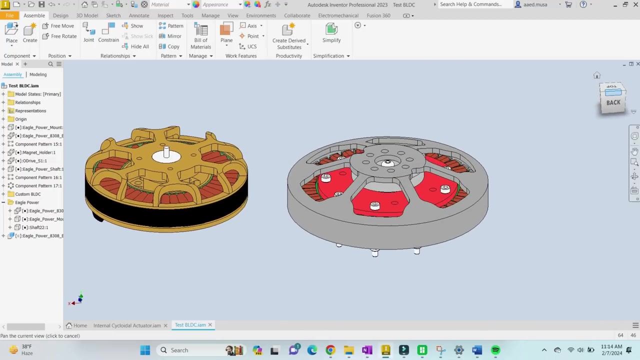 which is great. to make sure that i did the test properly. i also found the experimental kv of the eagle power, which i calculated to be 108, which is not quite 90 as the manufacturer claims, but it's close enough to know that my testing has some credibility. both motors are rated about the same. 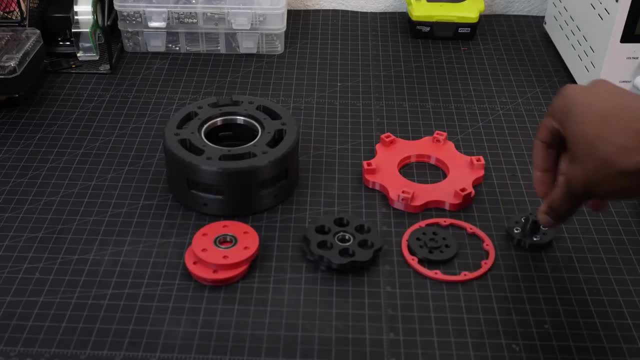 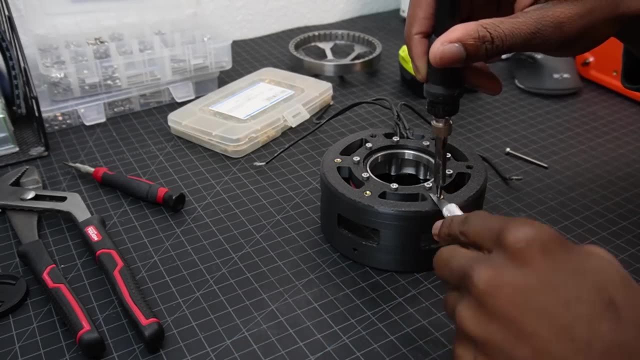 Finally, it's time to assemble the actuator. The stator is going to be part of the actuator housing, so I'm mounting the two together. I added threaded inserts to the top and bottom of the actuator housing to give me different mounting options. 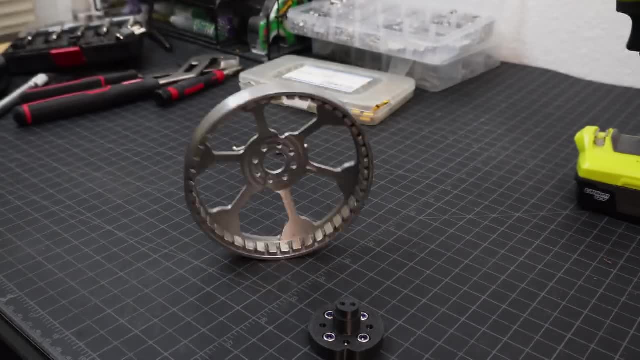 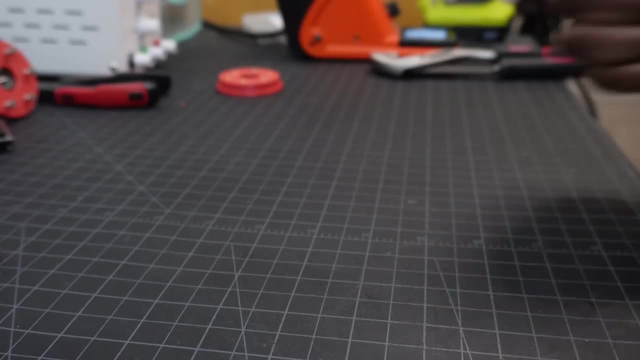 Now it's time to build the gearbox, which will essentially be the same process as building the prototype gearbox. The eccentric shaft mounts directly to the rotor. I'm then boring out these M3x5mm spacers to distance the bearings. It's a lot easier to build the gearbox when the spacers don't have threads. 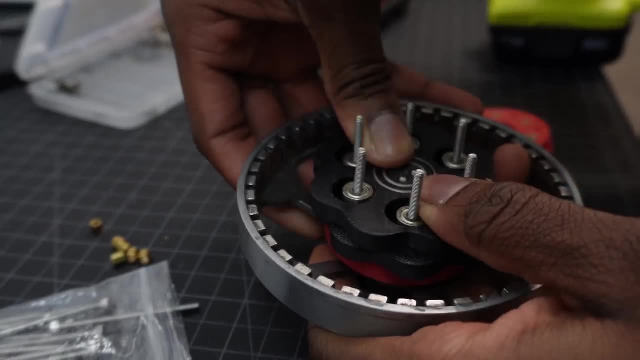 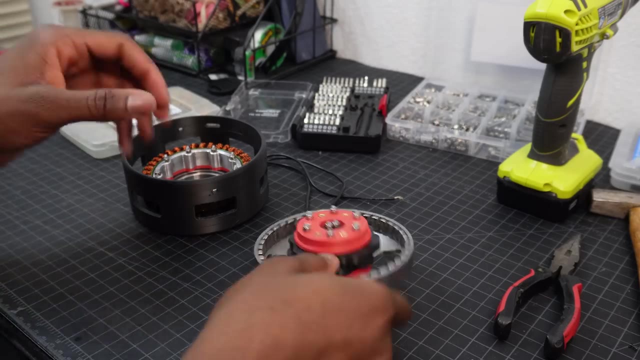 Building the gearbox is essentially a game of stacking with really tight tolerances. The rotor needs to fit into the housing, but because of the magnets it wants to lock onto the stator. Eventually, though, things do line up and it just pops in. 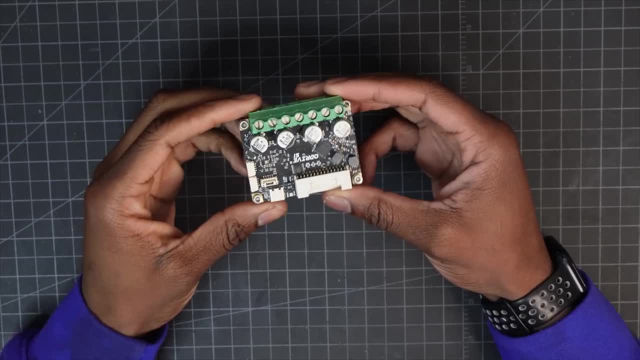 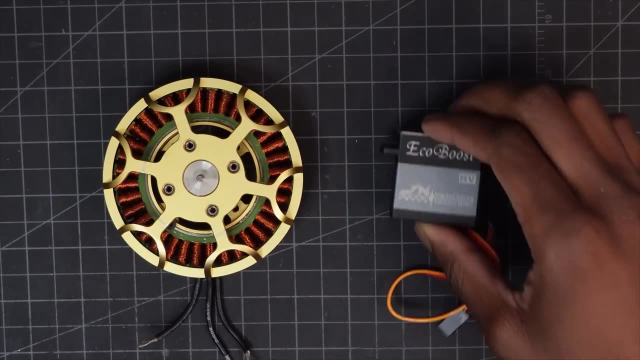 On the bottom of the rotor is an 8x2mm encoder magnet that's going to be read by an Odrive S1 FOC controller that has an onboard encoder. Think of this controller as a way to turn a brush's wheel. You can turn this motor into a servo motor, except along with position control, you also 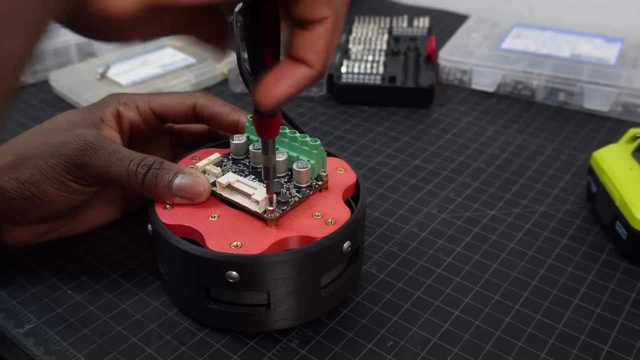 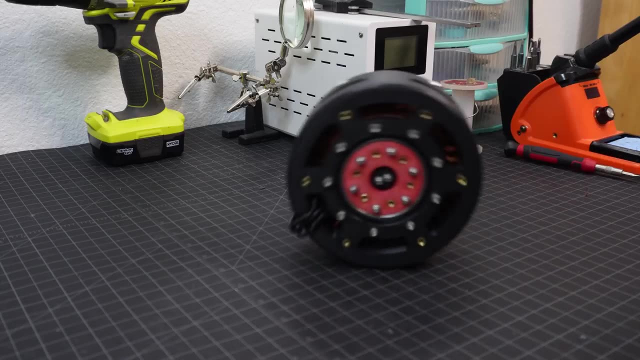 have velocity and torque control. FOC controllers are essential in robotics because they allow you to dampen or stiffen the actuator and software, which leads to more dynamic robots, And with that we have a one of a kind internal cycloidal actuator. 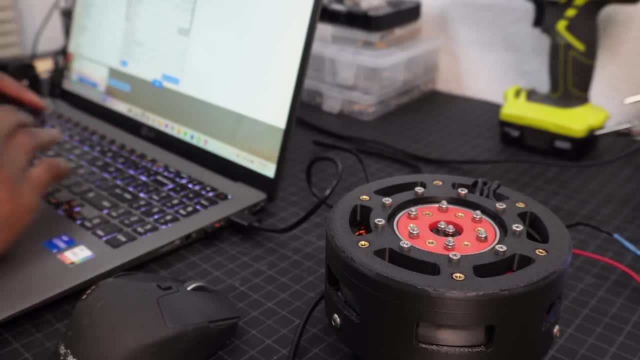 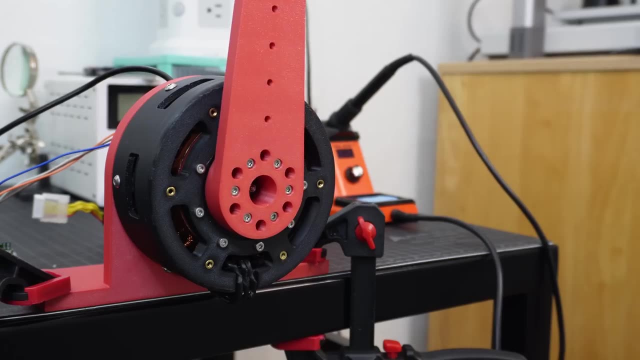 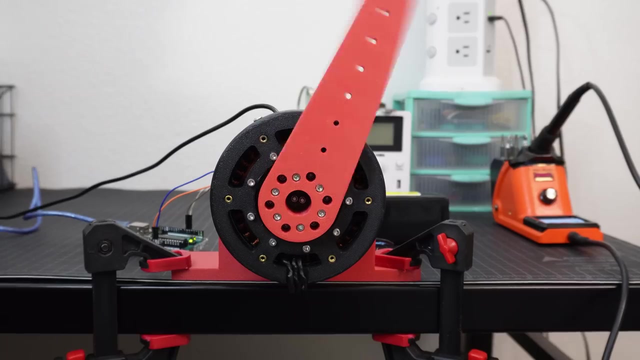 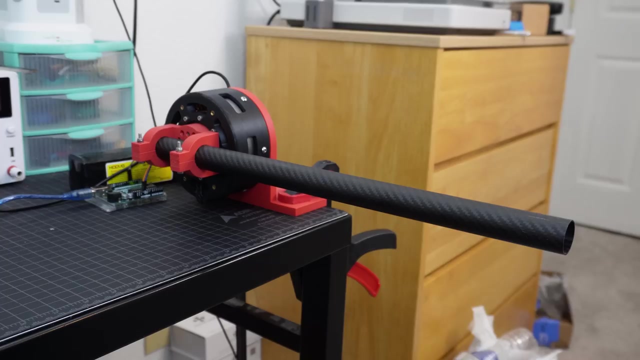 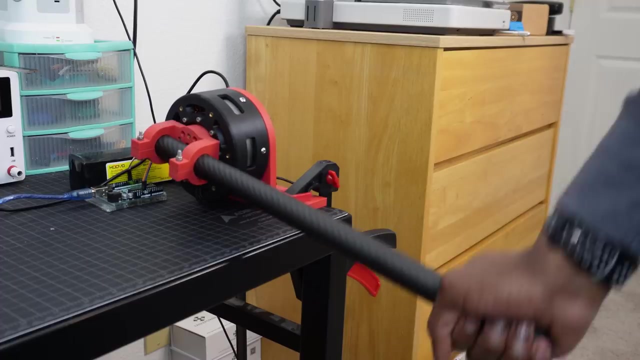 Now let's see just how well this performs. It's not perfect, but it's very easy to do. The motor is very easy to use. It's easy to turn and it's very easy to use. So if you're really going to do this, you'll have to be very careful. 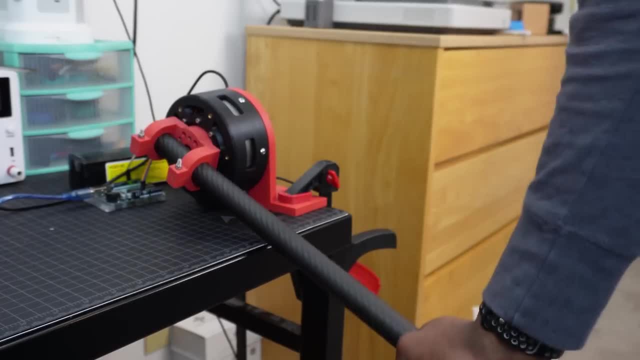 The motor will take a few seconds to turn, but it's going to do a lot. But if you're going to use it while you're on a ride, you'll have to be very careful. And with that we're done. Thanks for watching. 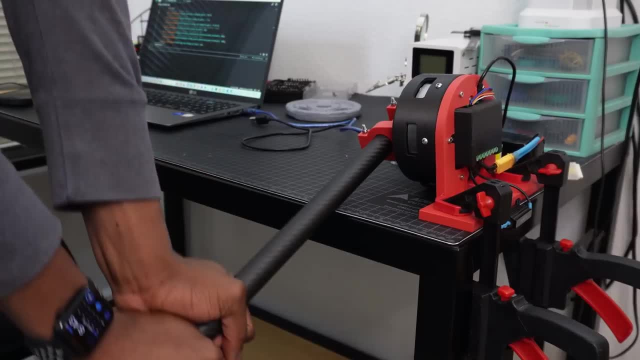 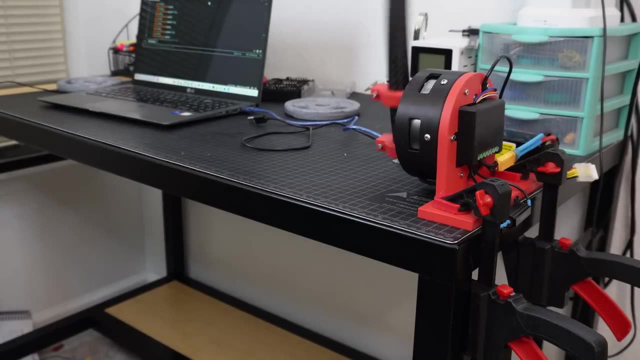 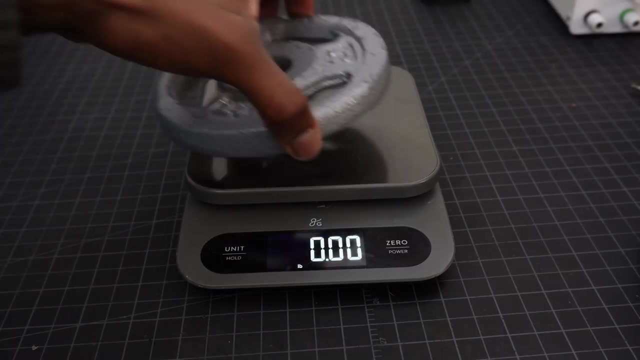 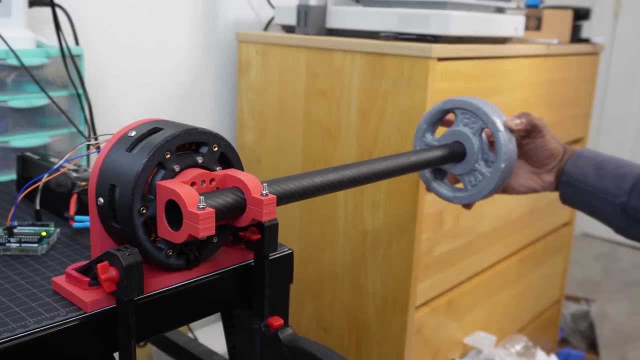 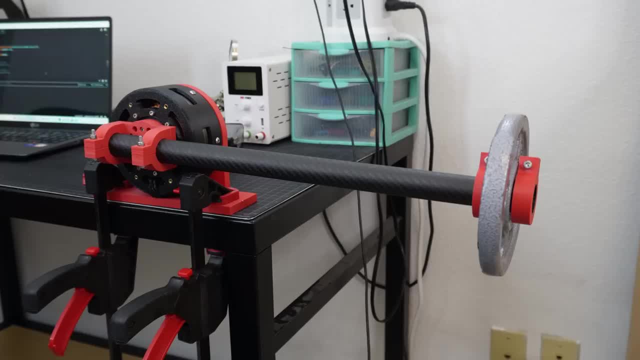 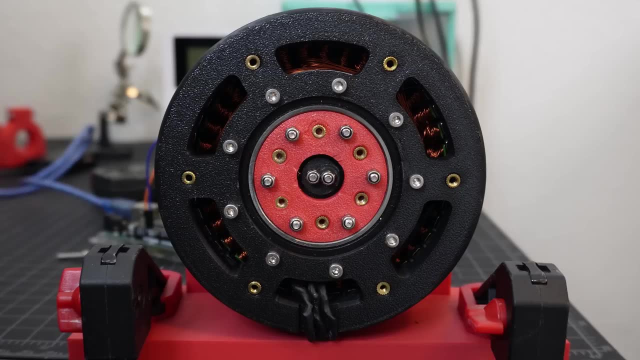 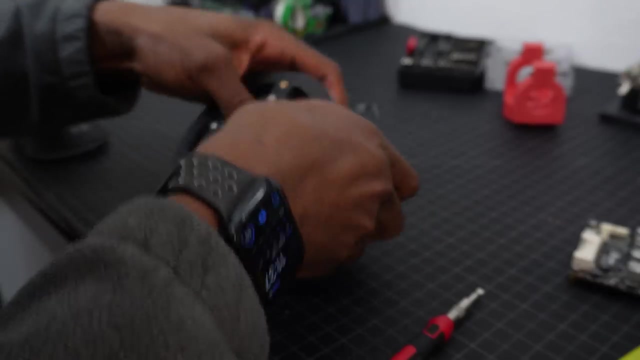 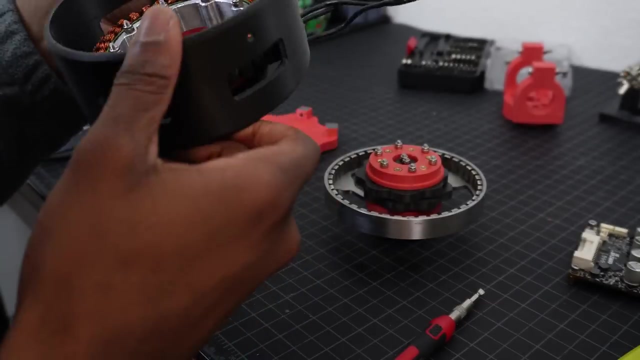 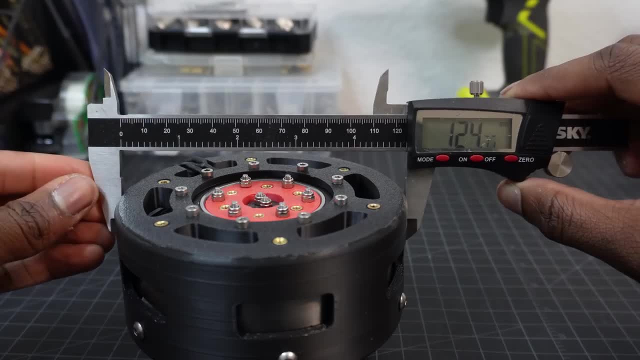 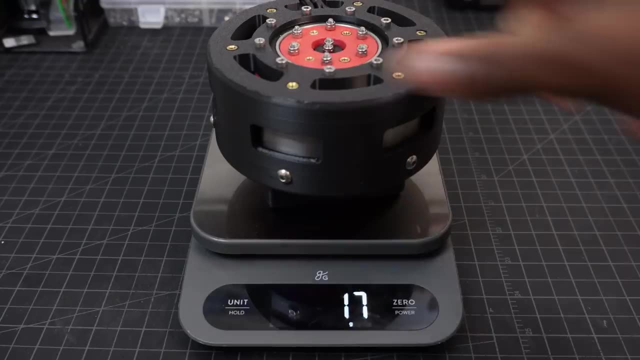 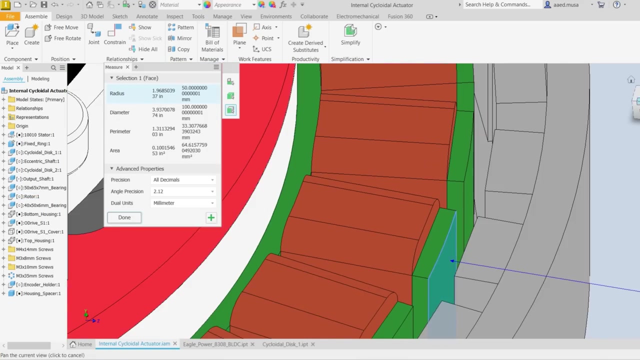 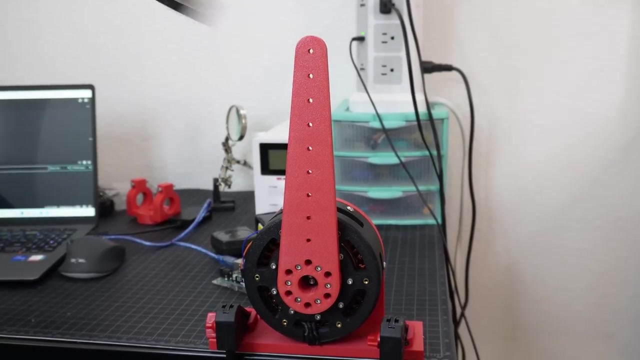 Now let's talk specs and results. The actuator is approximately 125mm in diameter, 84mm inrep and 1023g in weight. The air gap of the motor is 1.23mm. This is the gap between the rotor, magnets and stator. the smaller this gap is, the more flux it gets. The phase resistance of the motor is 75mOhm and the phase inductance is 41.0uO And yangs yang is 1.0.025mHg. 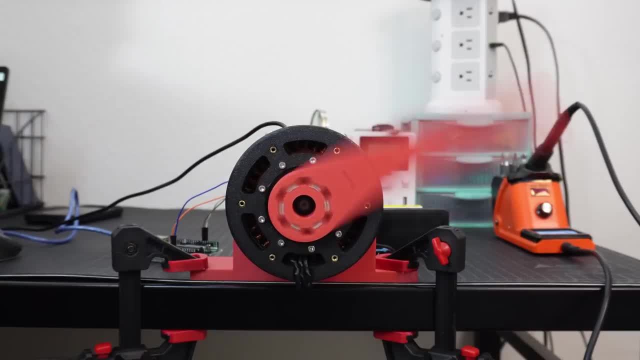 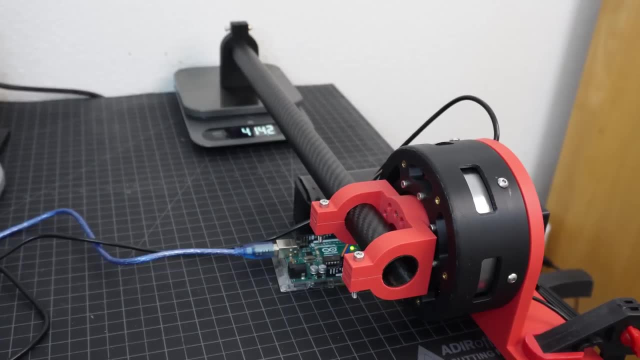 Now in terms of motor performance, the top speed on this thing is about 209 RPM at 22.2 volts. The max torque output is about 16.17 Nm. For reference, the planetary actuator that I made with the Eagle Power had a 9 to 1 reduction. 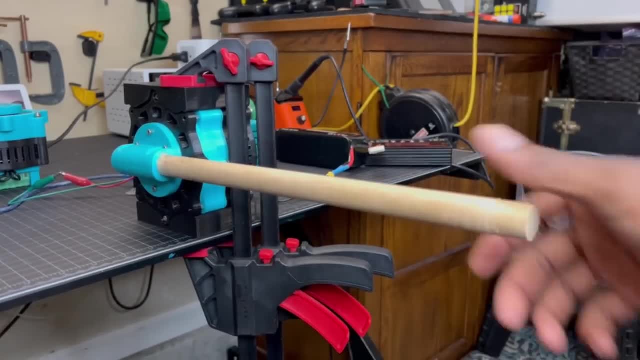 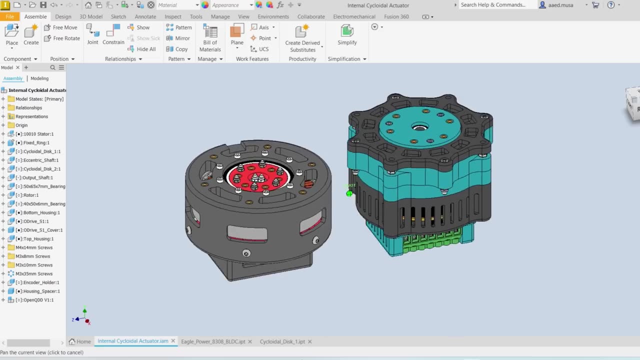 and a max torque output of 16.36 Nm, which means that both motors are essentially the same. As I mentioned before, the real benefit of this design is compactness. The internal cycloto actuator is about 0.9 inches shorter than the planetary actuator. 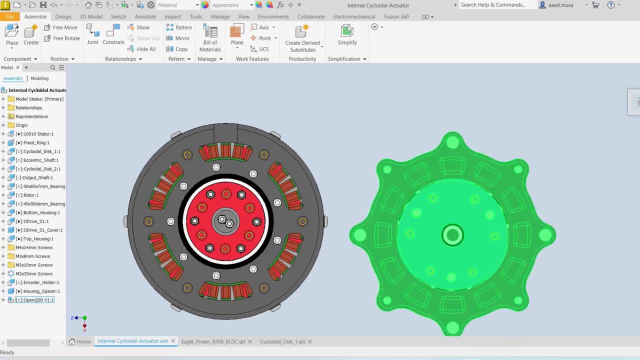 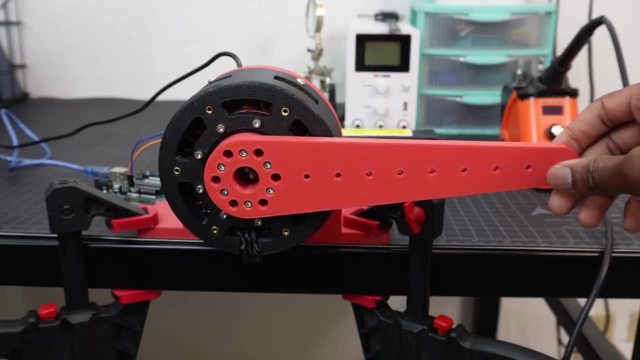 And if you ask me, 0.9 inches is a lot. I'd go as far as to say that 0.9 inches is more than enough. The backlash on the actuator was a lot more than expected. I think I could fix it if I worked on the tolerances more. 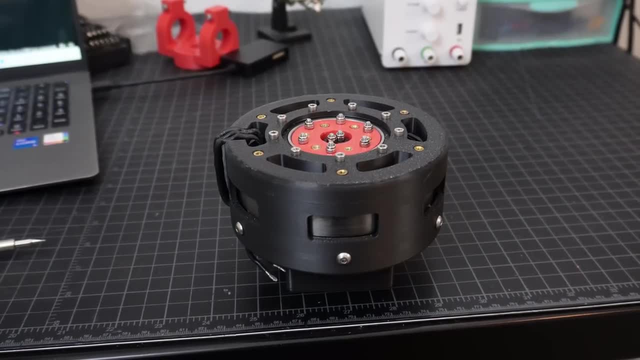 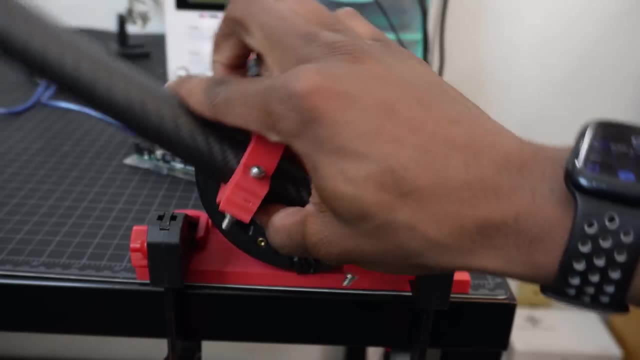 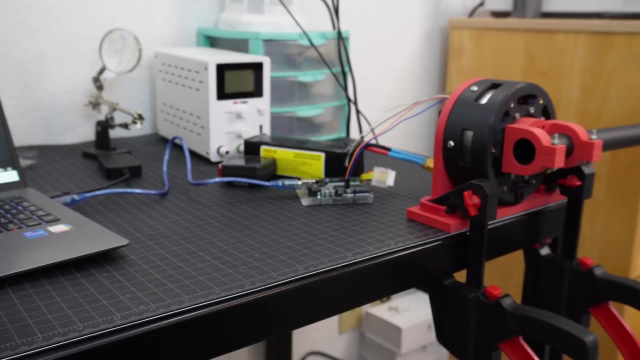 Now, at the end of the day, I don't actually plan on using this actuator for future projects. While this may be the optimal actuator, it isn't necessarily a practical one, At least not this version. It costs almost $400 to make, which is a lot more expensive than the Eagle Power actuator. 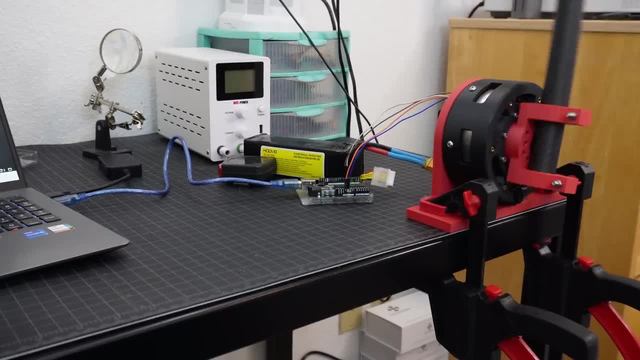 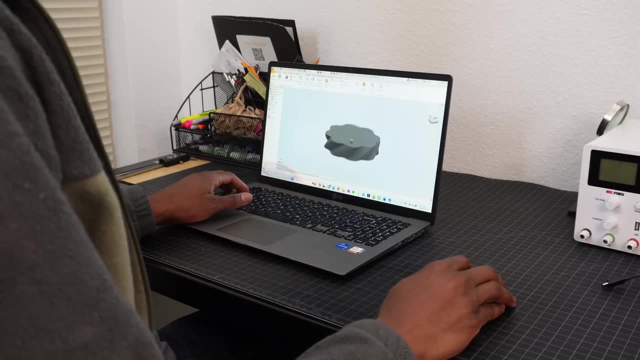 However, in the future I do want to make an even smaller version with the 81mm diameter stator fully out of metal. Now that would be awesome. This project also gave me a great idea for a future quadrupedal robot design. 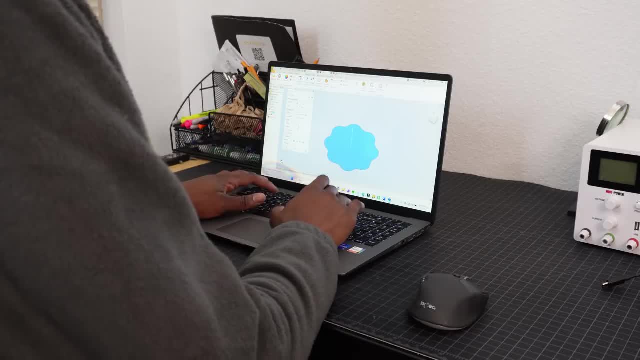 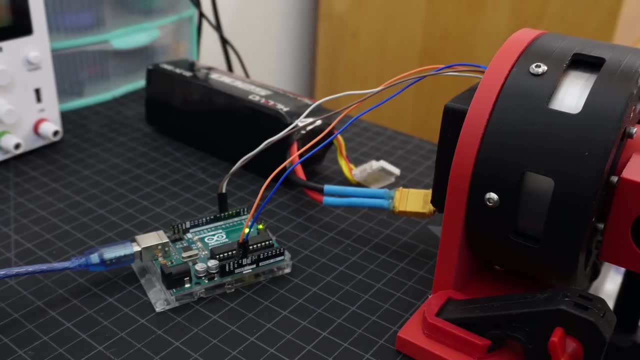 For me, this is the best part about engineering: You never really know if the thing that you make now will inspire something even better later. If you want to see those future projects, Be sure to subscribe to the channel. This project is fully open source and you can download the CAD and BOM at the link in. 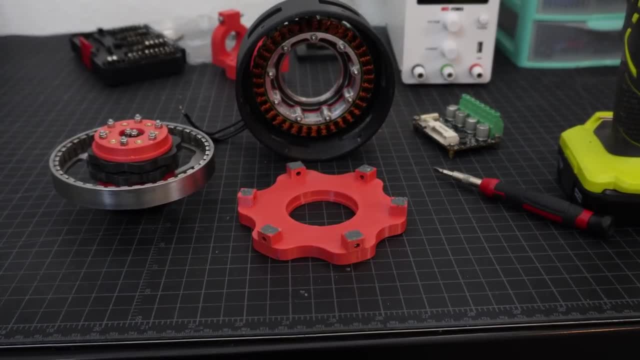 my description. That's all for this video. thanks for watching and see you in the next one. Uh oh.